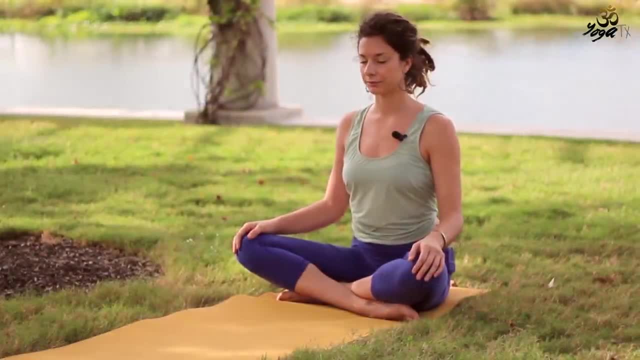 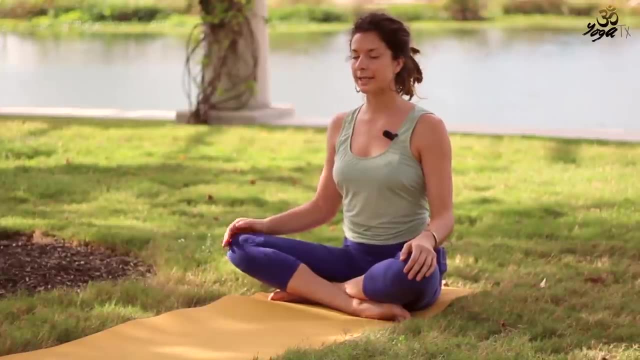 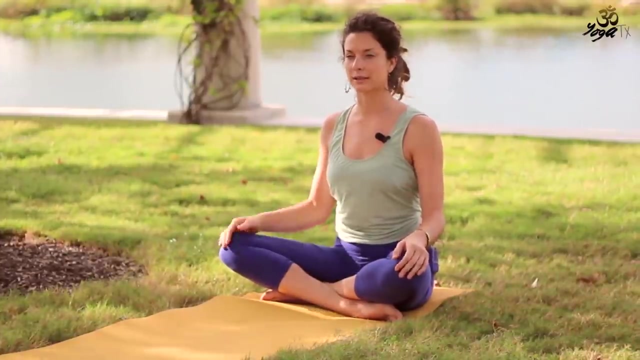 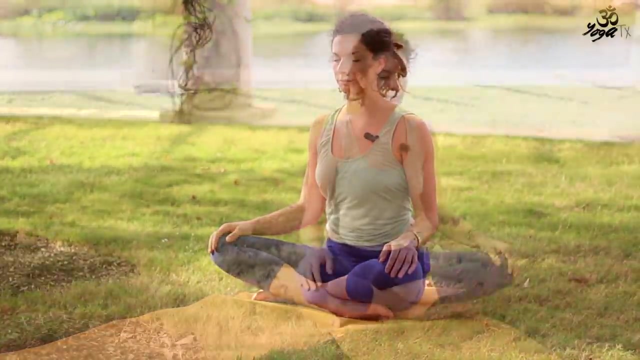 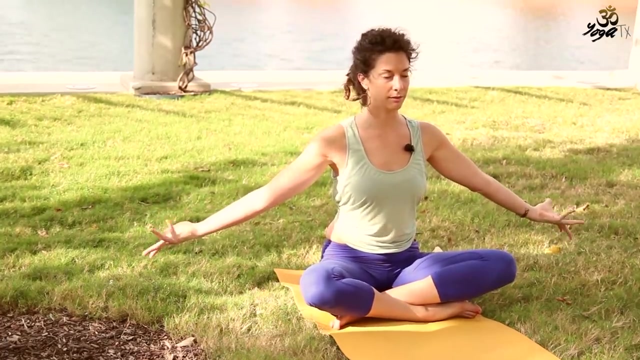 some inhales, Okay, And exhales, And see if you can match the two, like in for four, exhale for four. It has a calming effect And kind of come inward. Take your arms out, Okay, Palms to the sky And come all the way up And reach up. 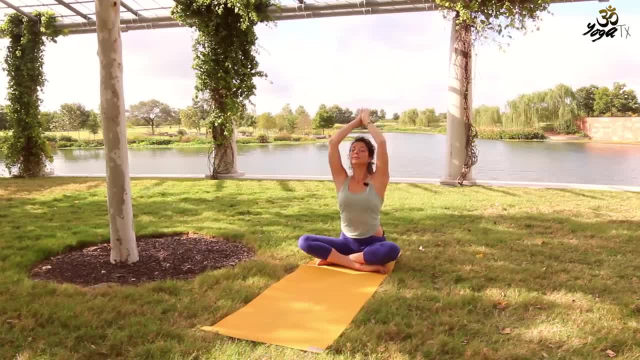 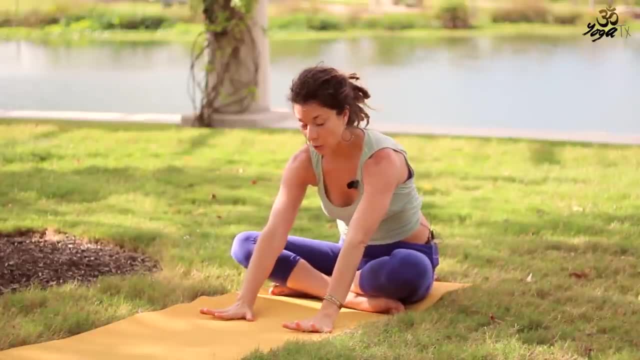 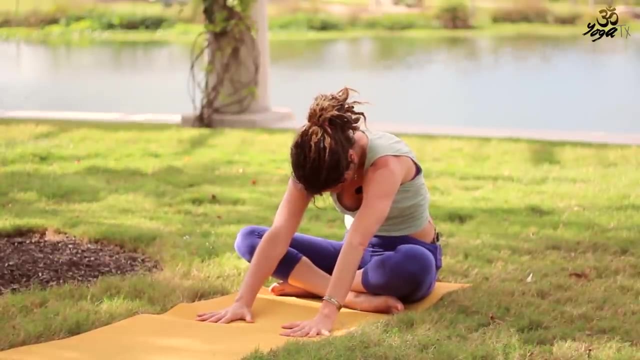 And go ahead and come to heart center here. Take your hands out front. We're going to push the earth away, So you're really going to round your back here And tuck your chin in towards your chest And then inhale, Feel like you're pulling your chest through, So 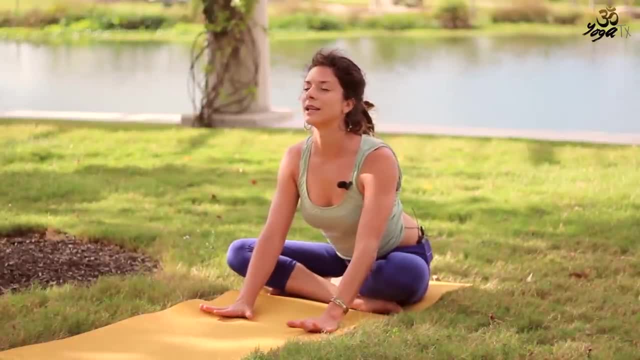 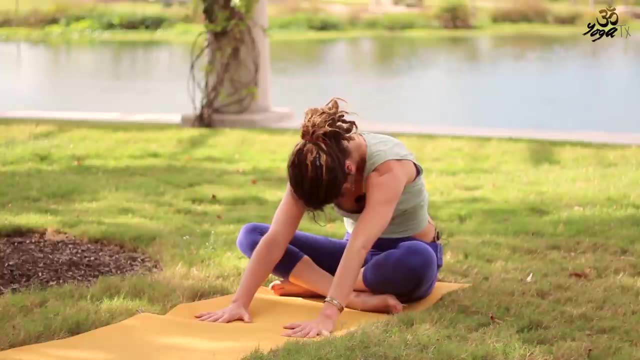 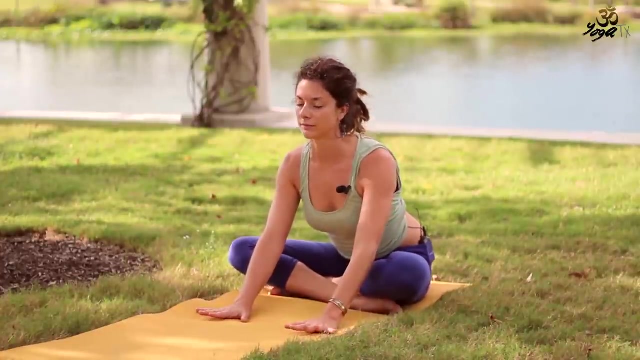 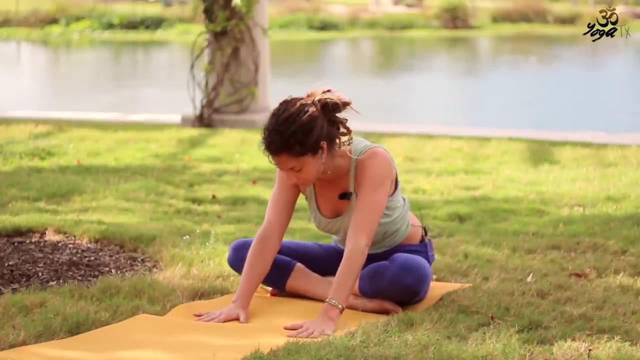 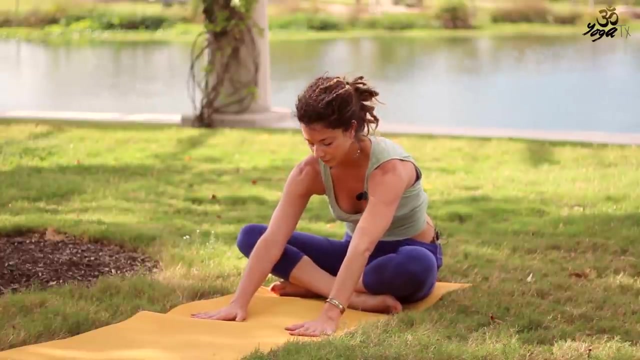 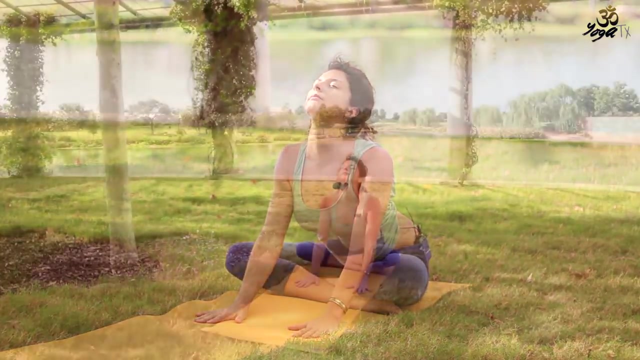 shoulders, back, Head up And then exhale, Push the ground away. Inhale, Come back through. It's warming up the spine. Inhale One more time, Okay, more time. Come back through, Come back up to center and take your right hand and place. 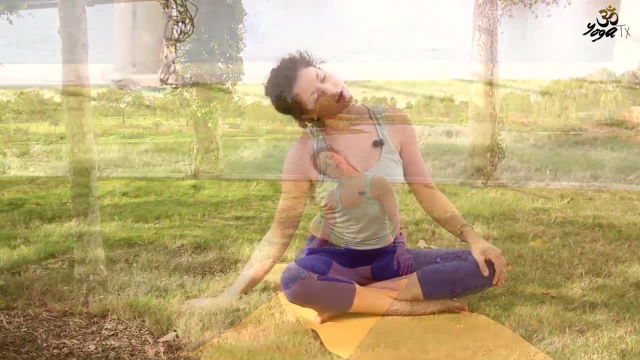 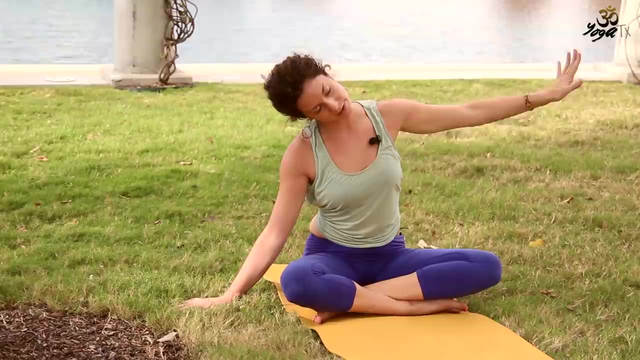 it over to the side here. We're going to lean over to our right hand and take our left hand out. You're going to tilt your head over to your shoulder and start to place your left hand down here, and it's really going to get a strong stretch right through here. So it might. 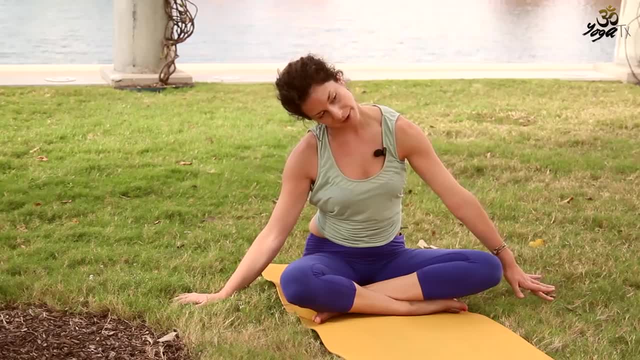 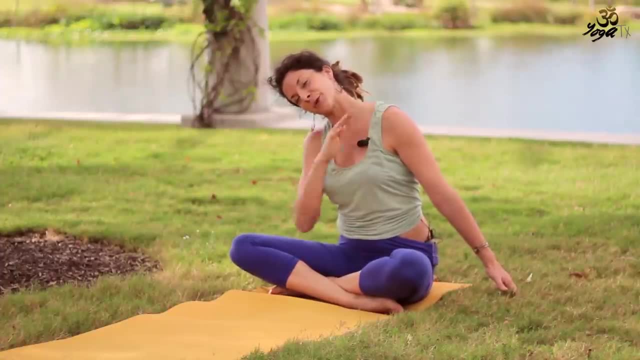 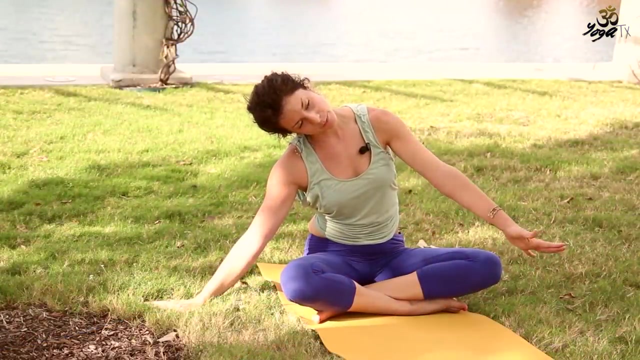 not touch all the way to the ground. You can play around with having it a little bit forward, a little bit back, but this is really going to open up this side of your neck and your shoulder right here, And you can come as far to the right as you need to. Sometimes I like to kind of move. 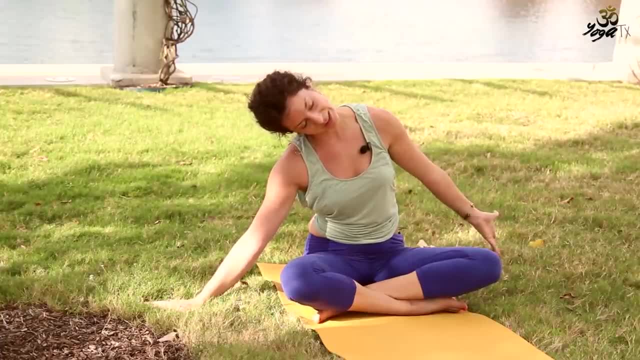 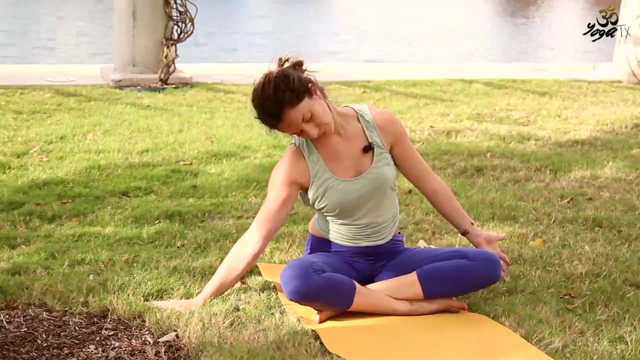 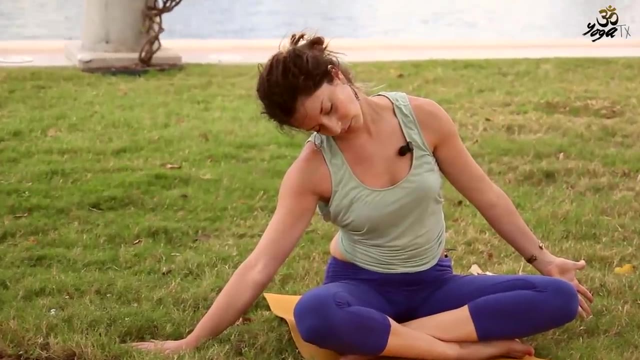 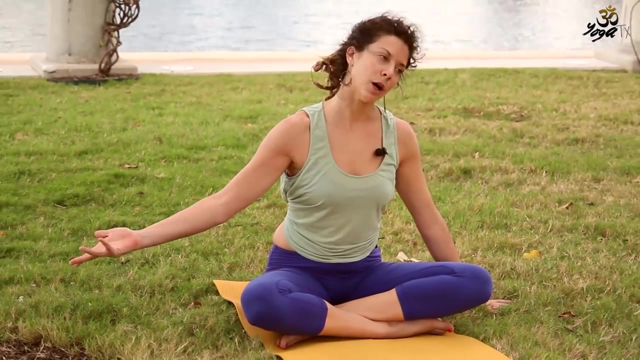 it. move it around here to get different little nooks and crannies. You can tilt your chin towards your chest. It's a really deep stretch. Come back up and we'll do it on the other side. So palm up and lean to the left. 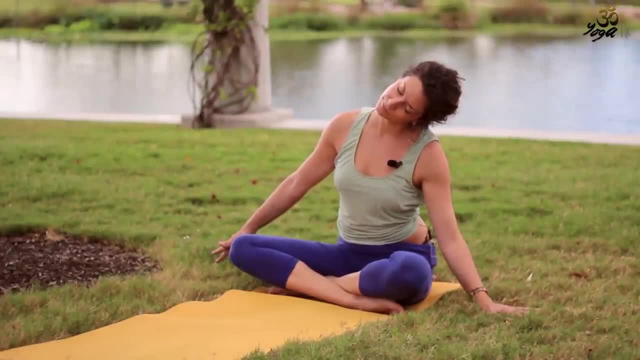 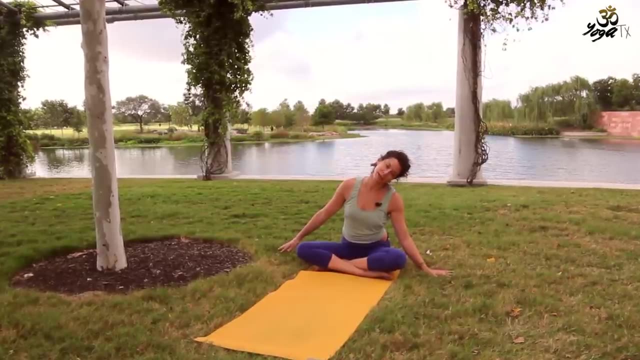 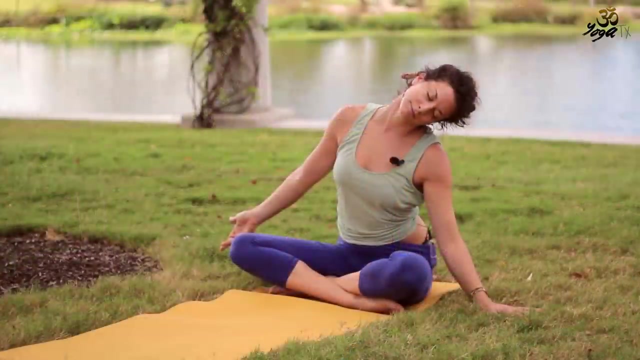 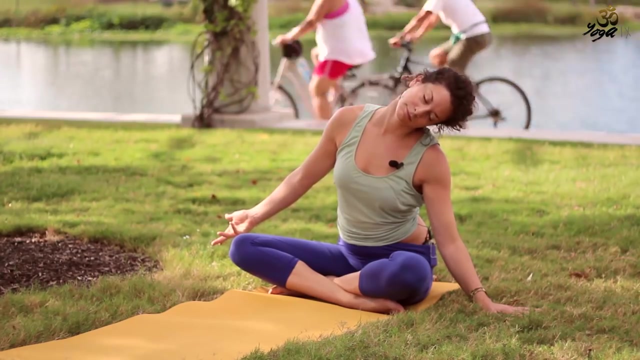 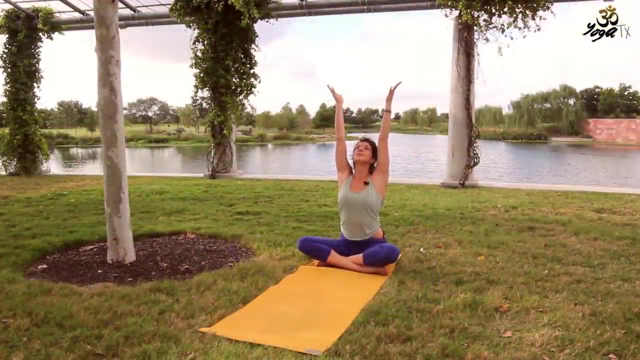 We'll start finding that sweet spot. It's a really delicate little muscle that can be intense, but it's very necessary to have them lubricated and functioning. Inhale, come back up. We'll come, go all the way up. Look up to the sky and take your right hand to. 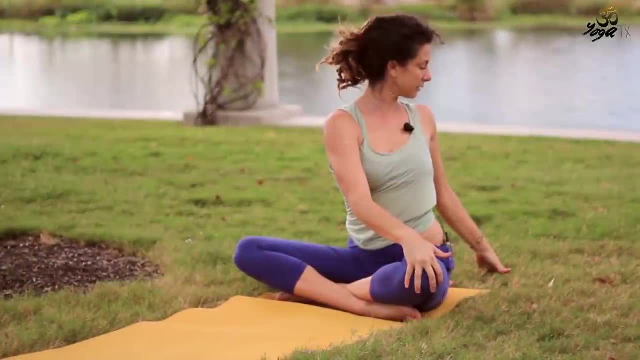 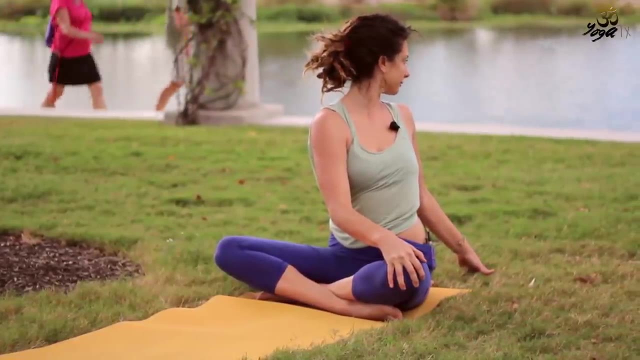 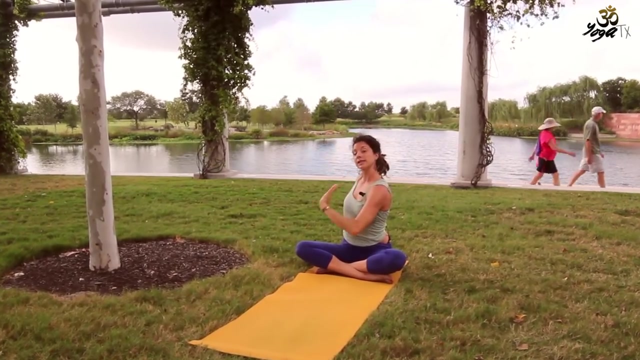 your left knee And we'll exhale and twist And then take an inhale and an exhale here. Look over your left shoulder And come back up to center, Inhale and then exhale, twist left hand, right knee. 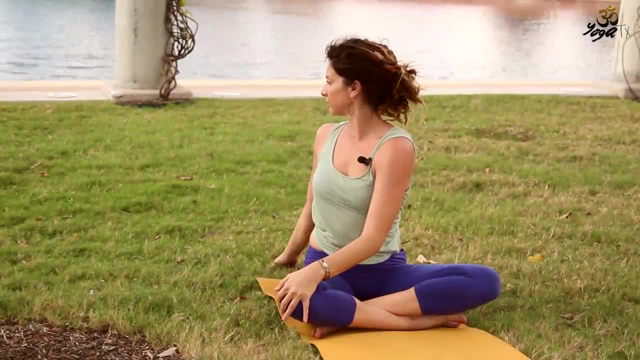 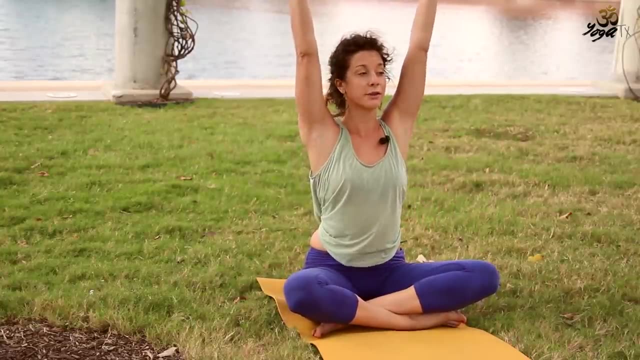 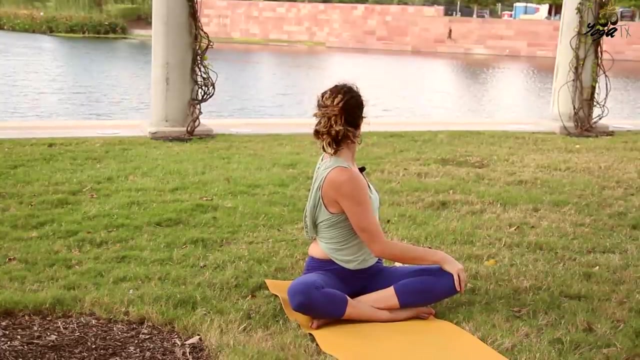 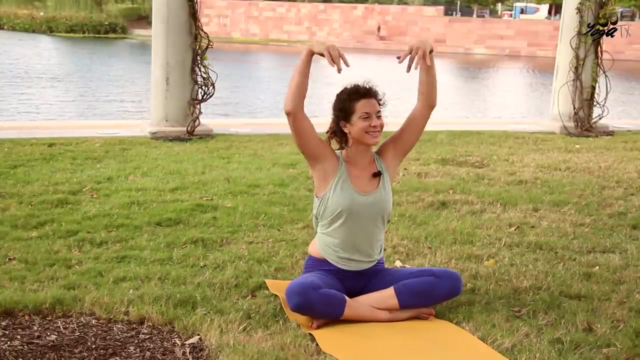 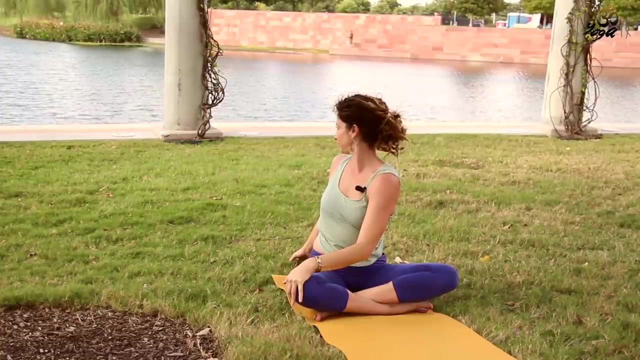 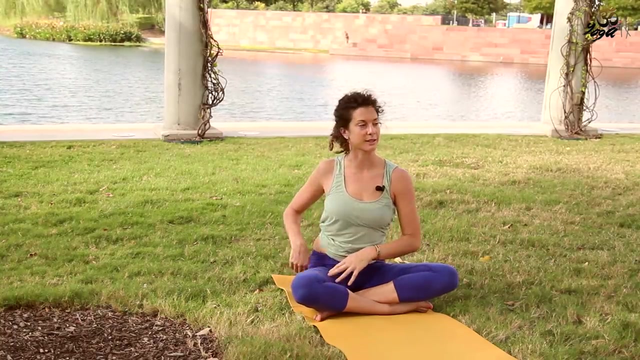 Take a full breath cycle here, Back up to center. When you're twisting, twist your head left Last, sorry, So twist your body and then bring your neck around. I'm gonna go one more time to the other side And back to center. 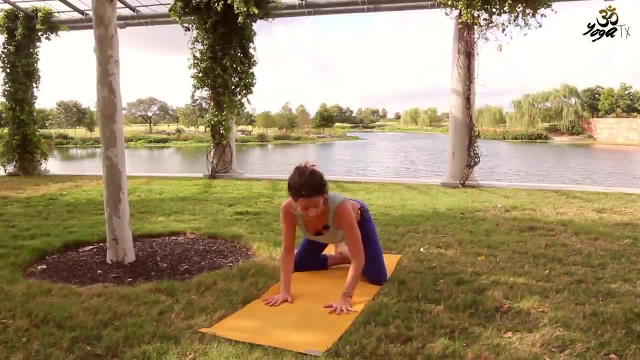 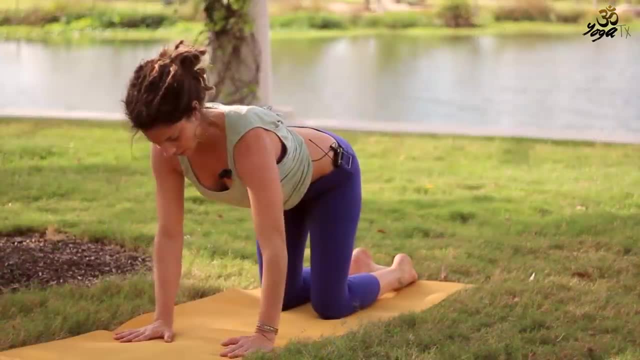 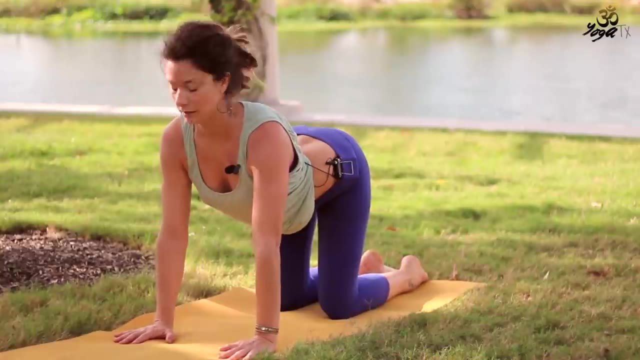 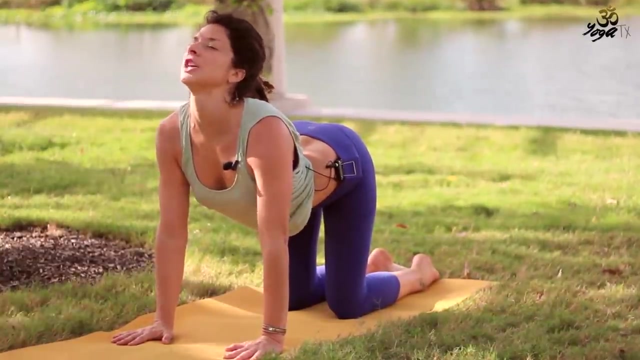 Take your hands and we're gonna roll forward over our knees into tabletop. So just come forward and tuck your toes here. We're gonna take a cat-cow variation. So we're gonna take cat here. So tuck, untuck, bring your hips up, arch your back, chin up shoulders on your back. So this is the cat. 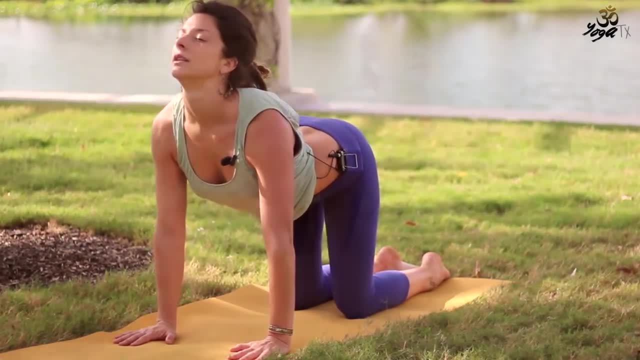 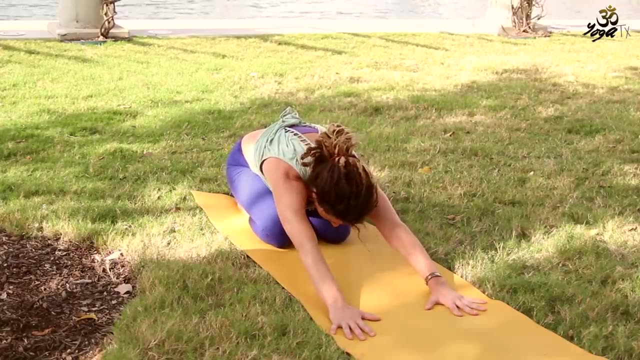 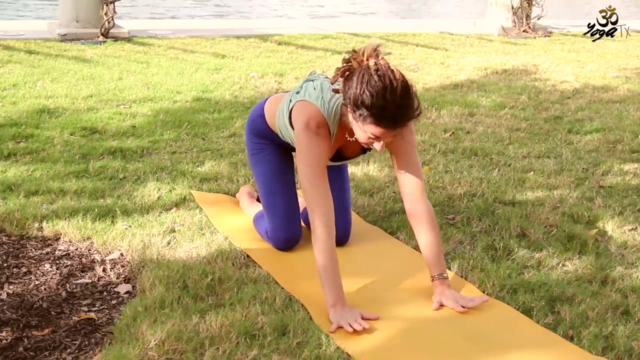 Push the floor away, Then on your exhale, we're gonna sit back on our hips. So push the ground away and sit your hips back onto your heels as far as you can. So inhale, come up and arch, And then exhale, come back. 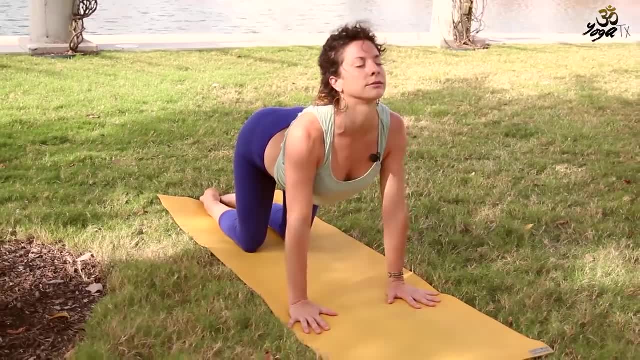 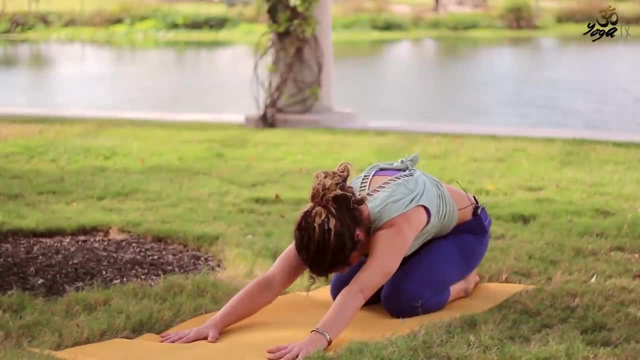 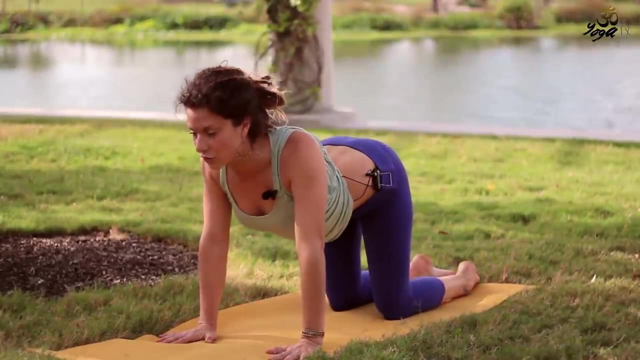 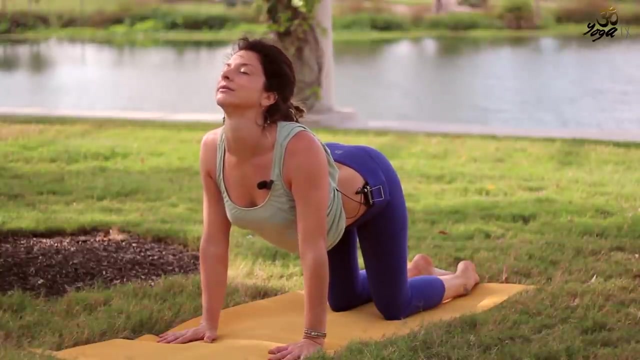 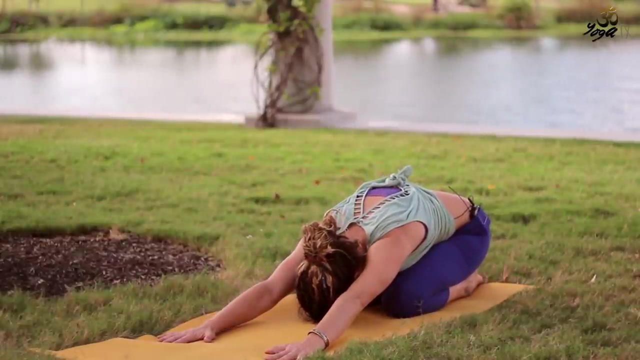 Inhale up and arch and exhale back. Inhale up and arch. Make sure you push your shoulders away from your ears. You don't want them like this. You want to push them back onto your shoulder blades and then back. 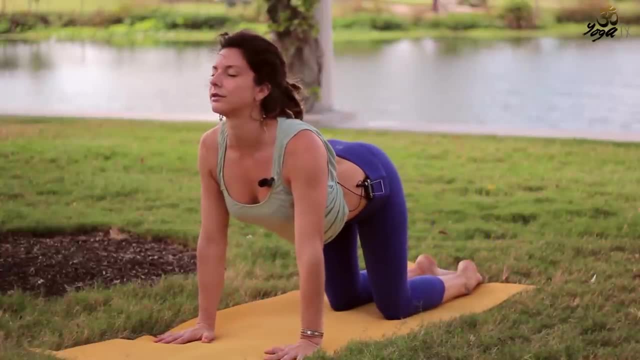 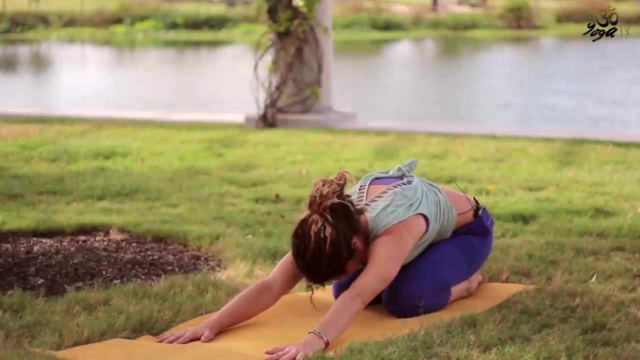 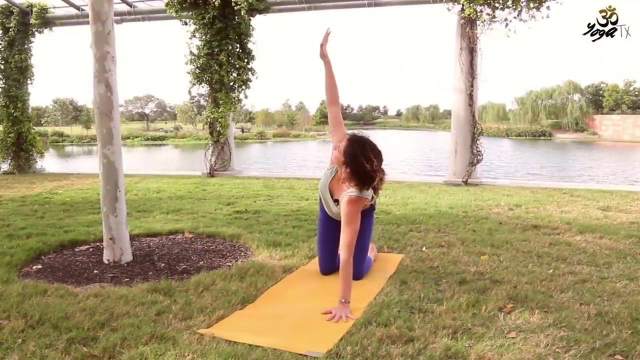 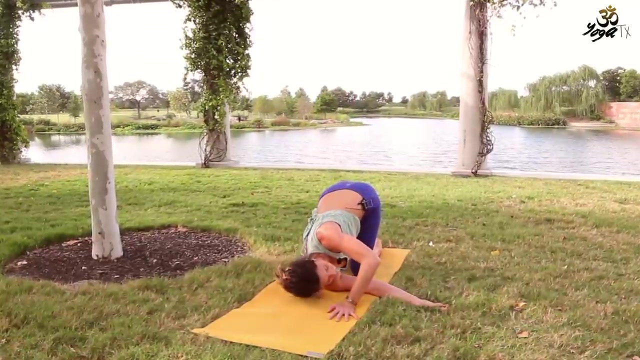 Inhale up and arch and back. Come back to tabletop. Take your right hand up, Twist as much as you can right here and look up. We're going to thread through. If you'd like to, you can put your leg out here. 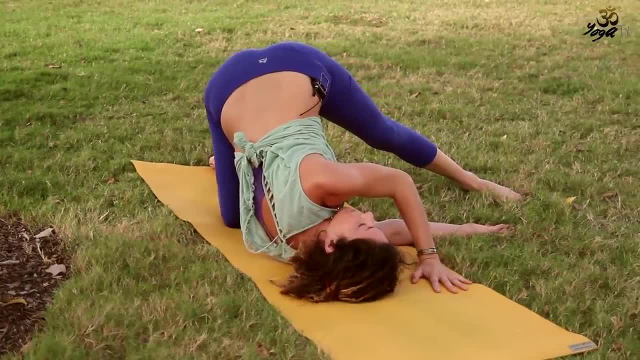 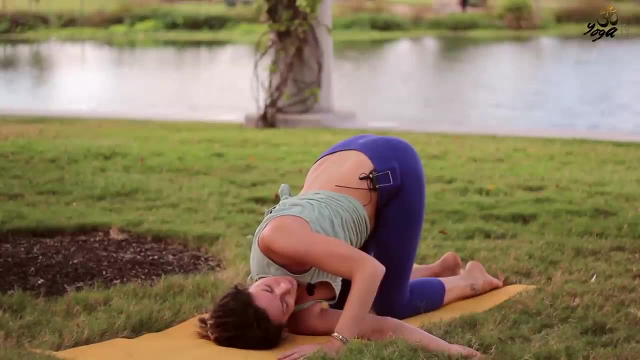 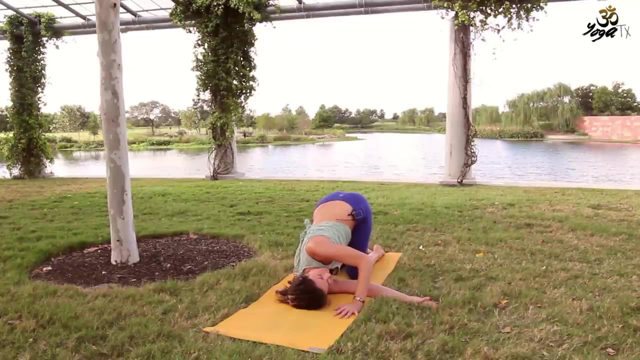 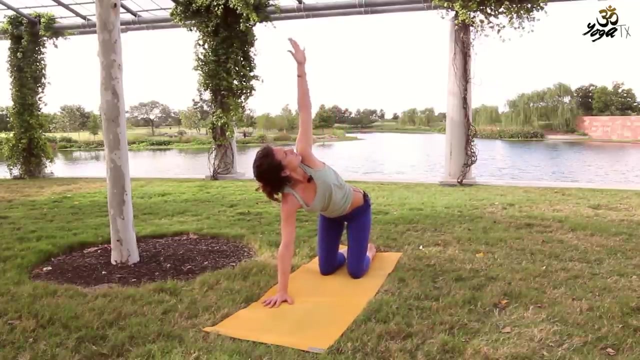 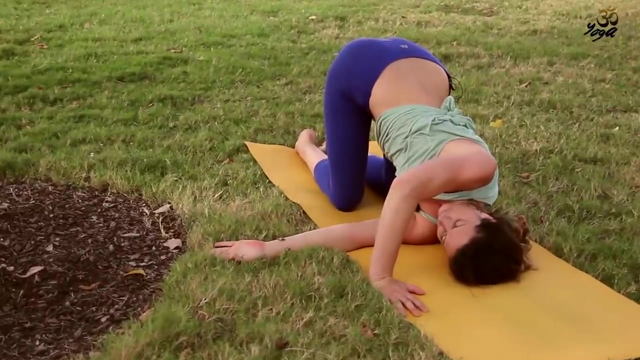 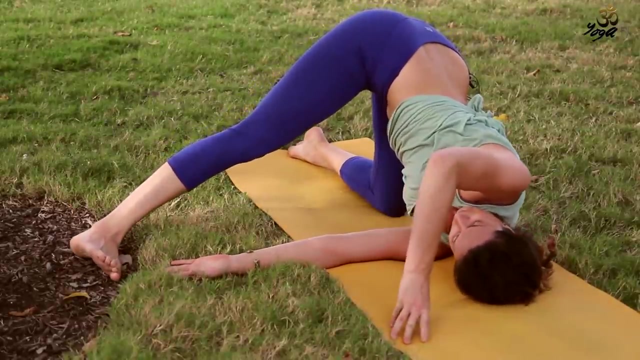 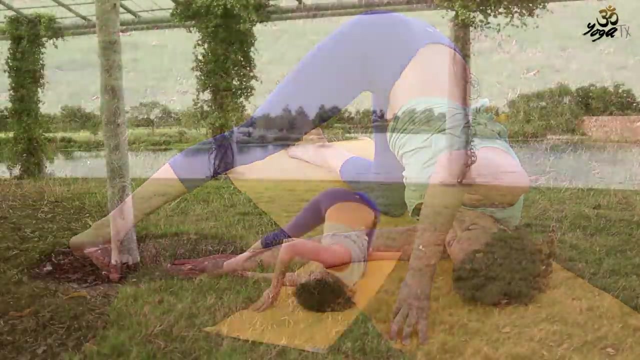 This will help you twist a little bit more. You can also leave it right here as well. Good, Good, Good, Come through, We'll do it on the other side. Good, All right, That was really fast. Awesome, I'll see you right here. 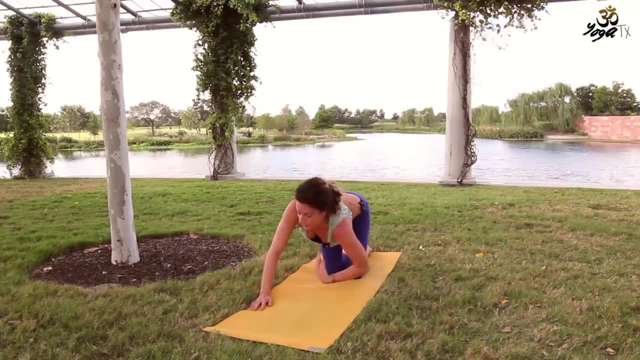 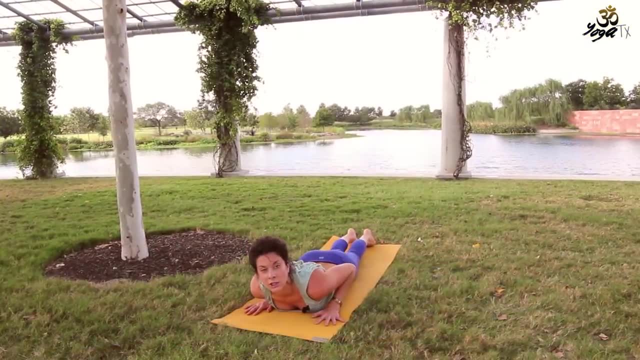 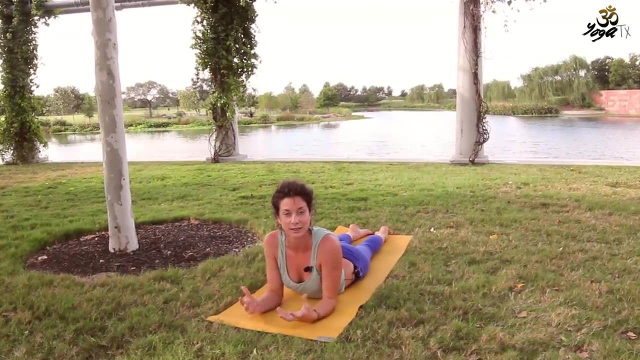 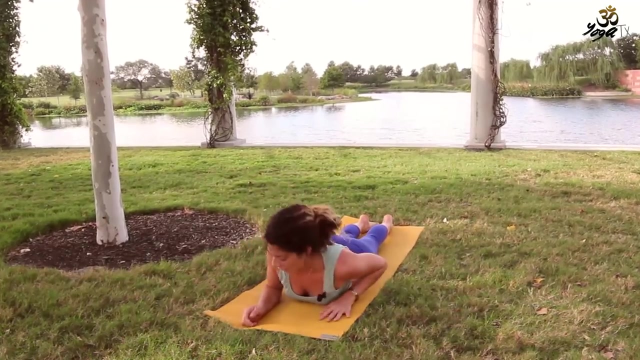 We're going to come all the way down onto our mats. So a lot of times back pain is caused because there's weakness in the back. So we're going to do a few back strengthening poses that will help keep pain from creeping in on you as much. 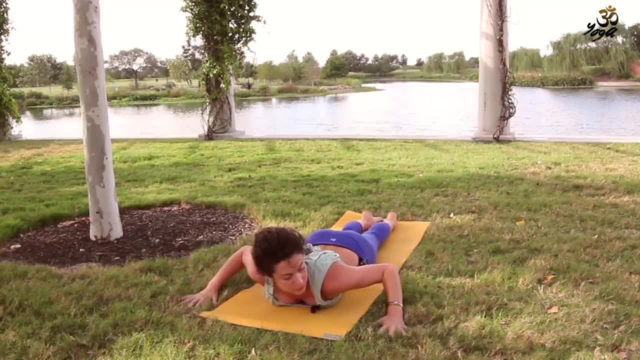 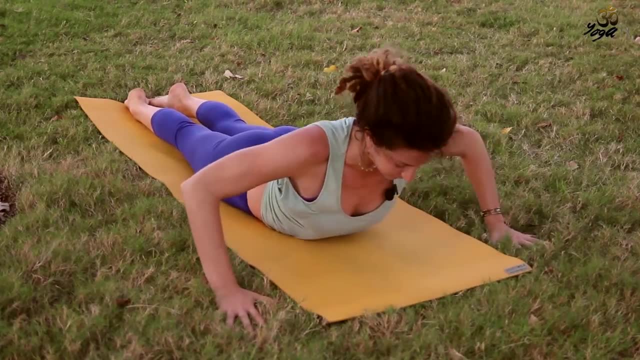 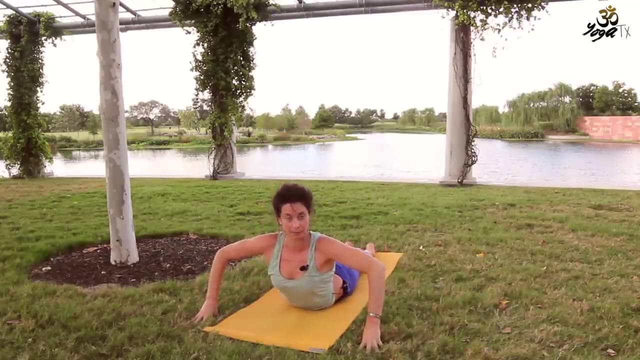 So come all the way down and we're going to actually bring our hands out to the side here. So a little bit off of your mat and bring your forehead to the ground and then inhale. you're going to lift up from wide here. Think about having your elbows up. you can come up on your fingertips as well. 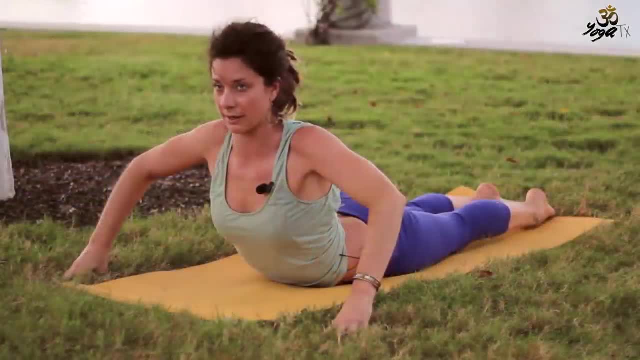 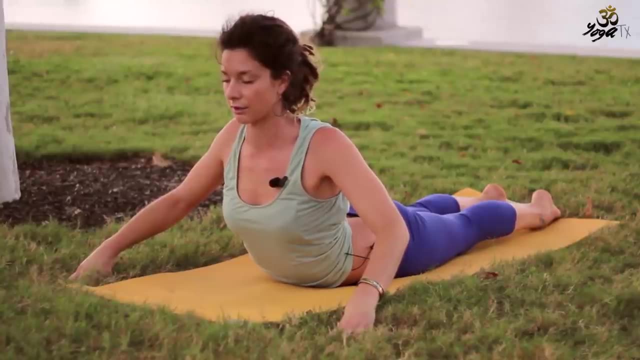 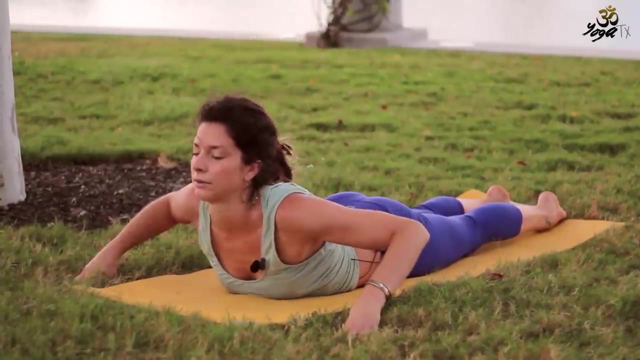 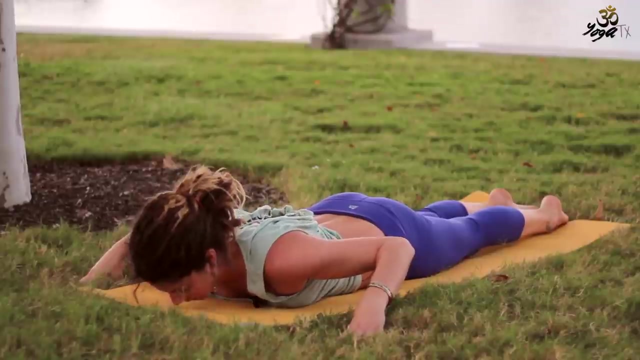 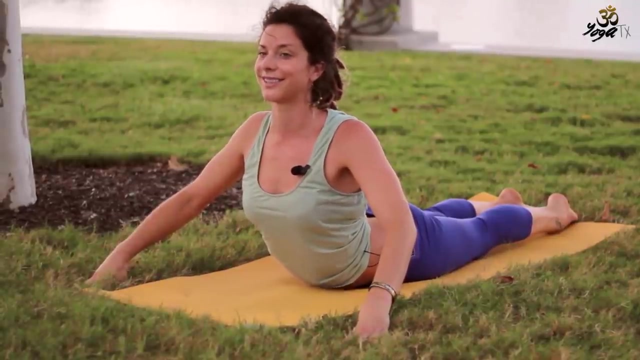 Your elbows up now roll your shoulders back, Bring your elbows in towards your chest. Feel that action. Try to come up a little bit farther here, Okay, And inhale and come down and go one more time in that variation. So inhale, rise shoulders back, elbows in, and lift up a little higher and look up and 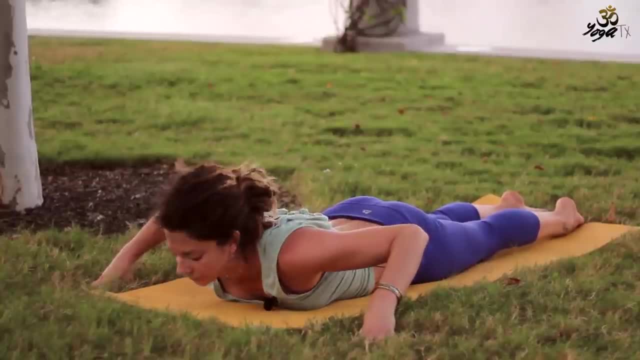 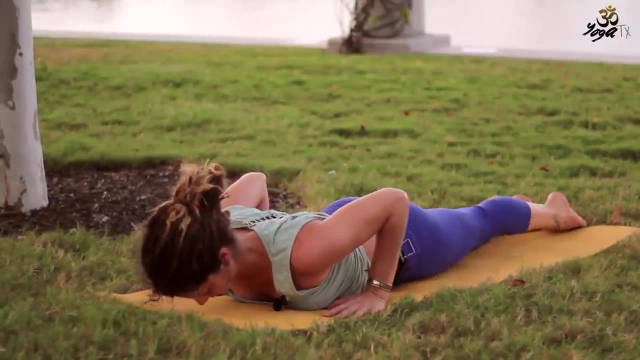 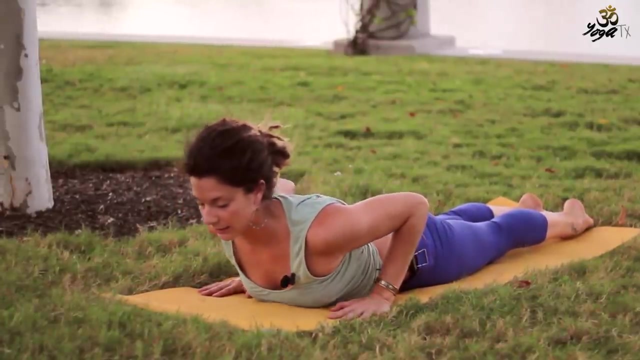 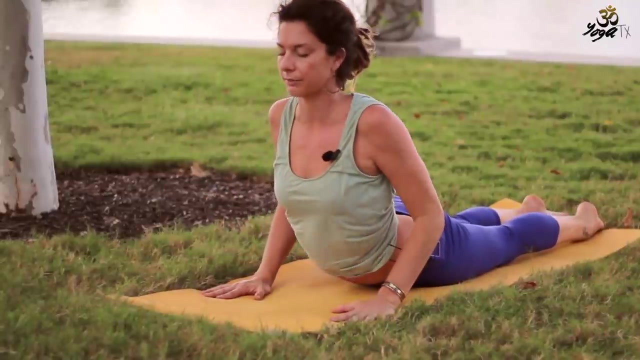 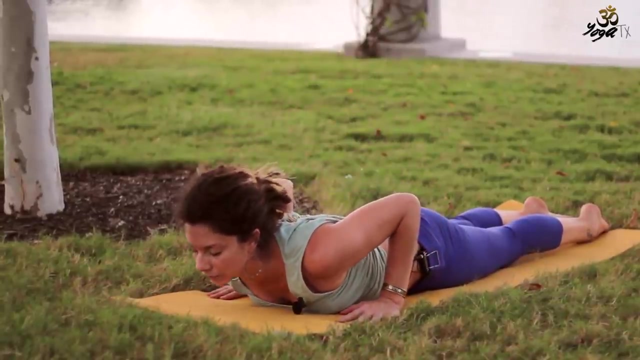 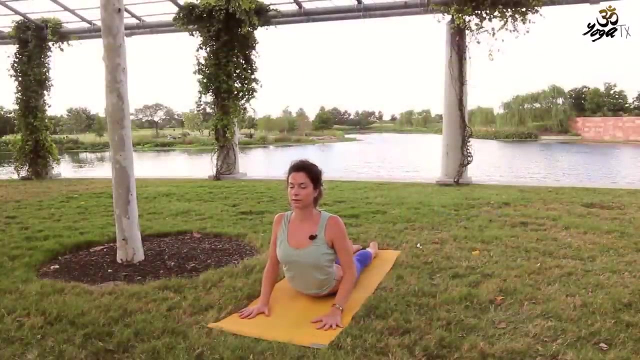 exhale down and bring your hands in And right next to your rib cage here. So inhale, come halfway up and exhale down And inhale. come up higher And exhale down And inhale. come up to your full expression. 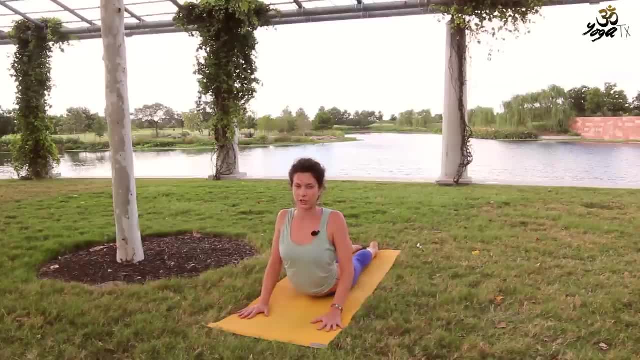 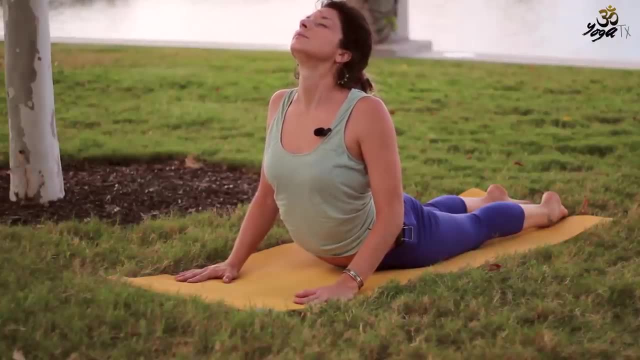 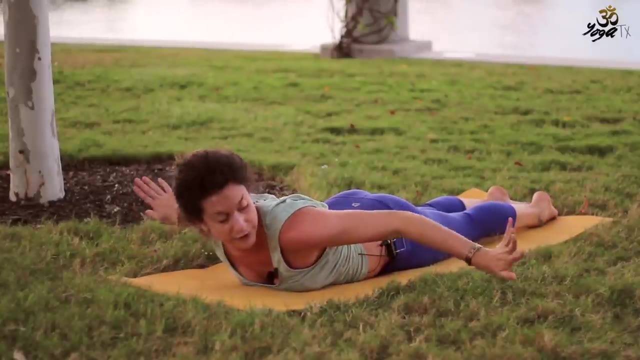 You never want to have the arms straight in this position in cobra. Head back and come all the way down. Take your hands to your side here. Okay, We're going to leave our head down and we're going to lift our legs. 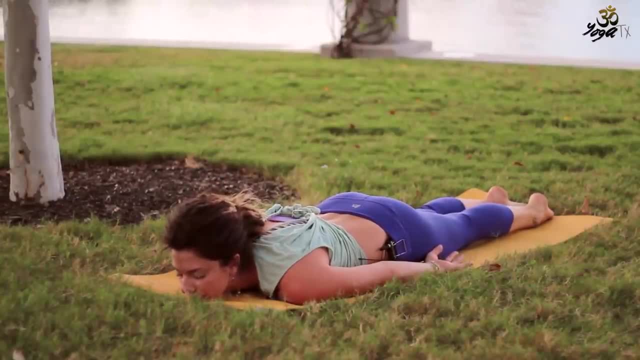 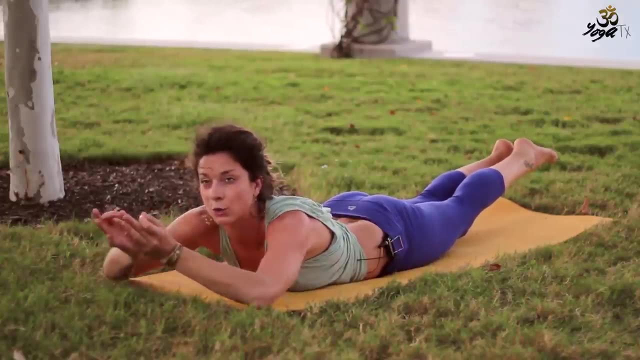 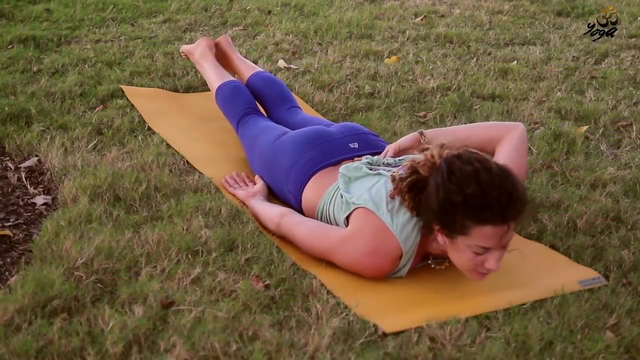 So you're going to rest your chin and on an inhale lift up, You want to bring your ankle bones in towards each other and try to keep your feet together if that's possible. So it's really targeting this lower back right here. 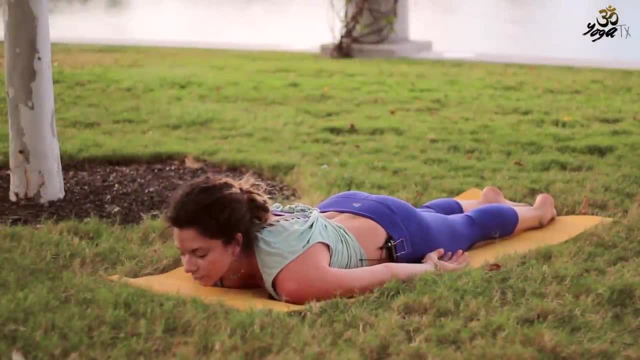 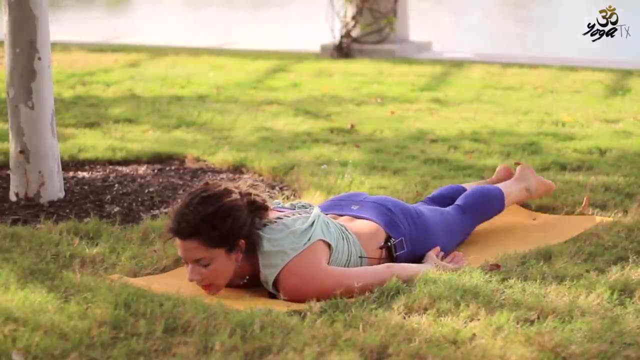 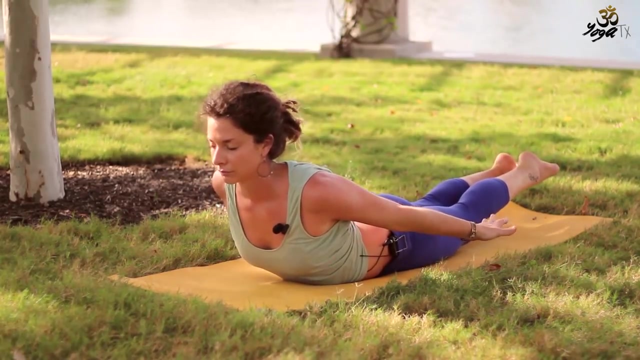 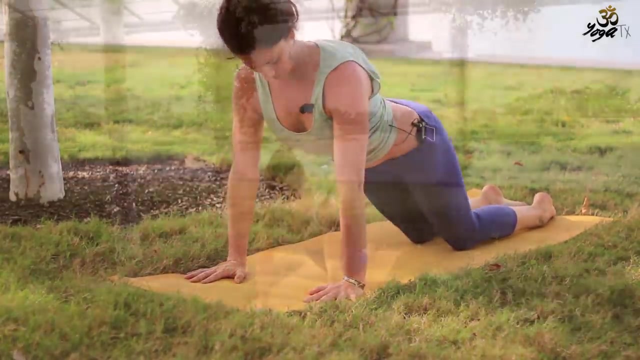 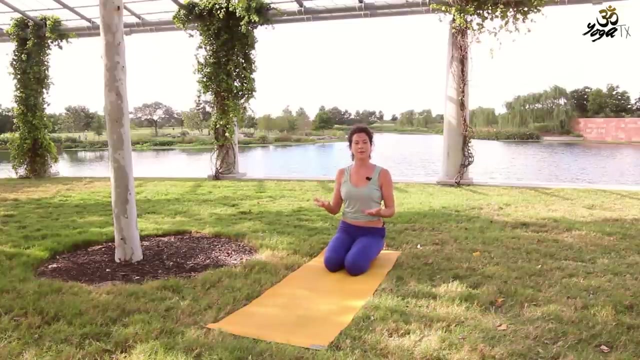 And lower down. Take an inhale and an exhale And one more time lift up. This time go ahead and lift up on both sides And exhale lower And plant your hands. Come back to sitting here, So we're going to do a little vinyasa variation. 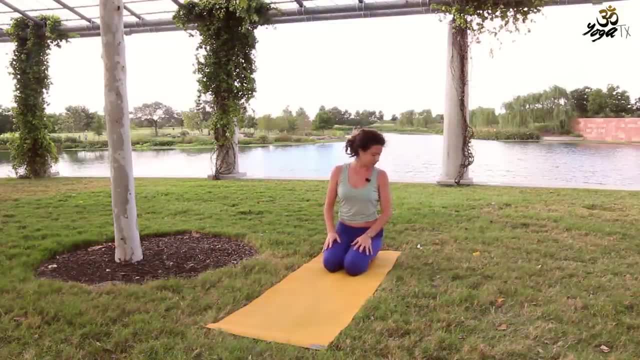 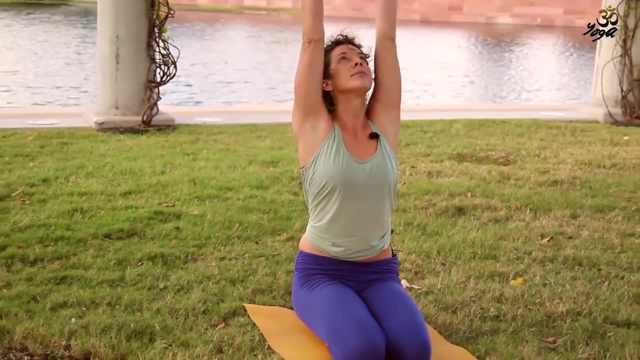 We'll be standing here, We're going to do a little vinyasa variation. We'll be standing here, We're going to do a little vinyasa variation staying on the floor here. So go on an inhale, lift your hands up, look up And exhale bring. 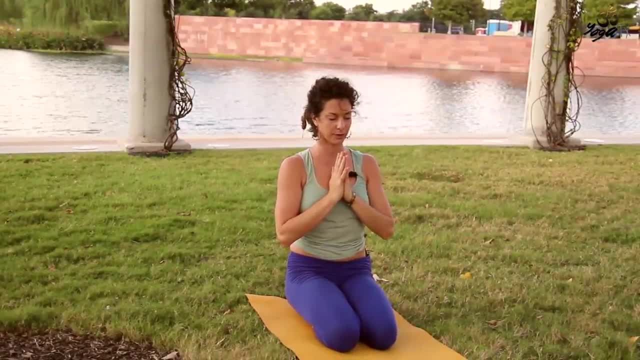 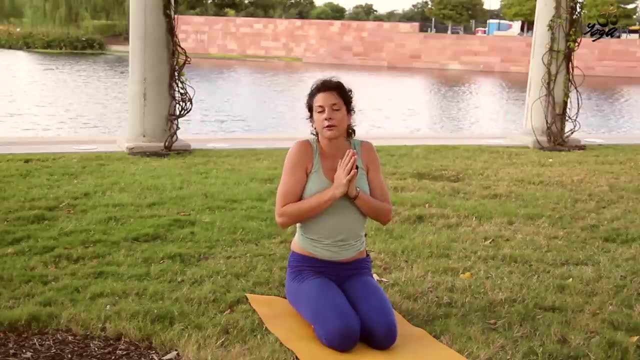 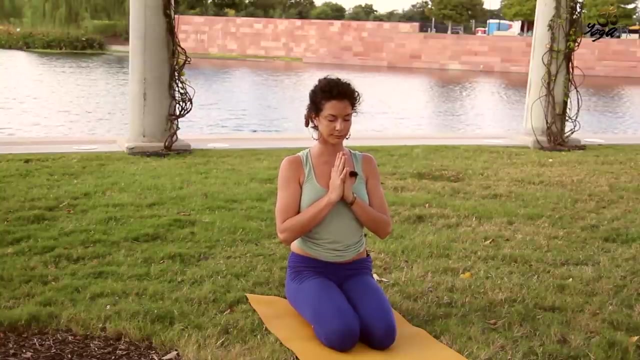 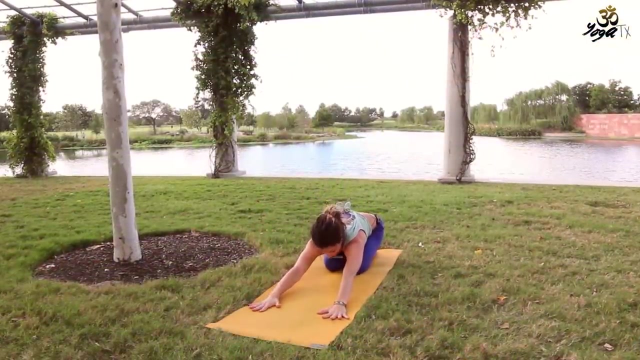 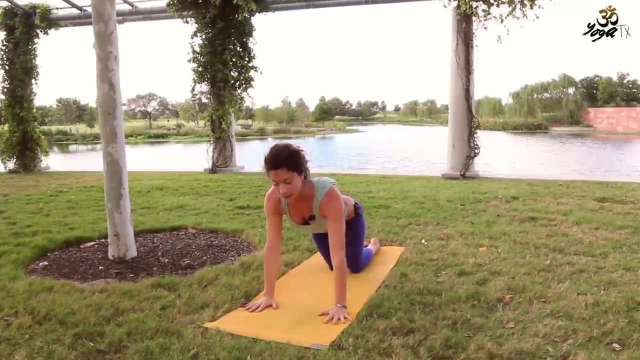 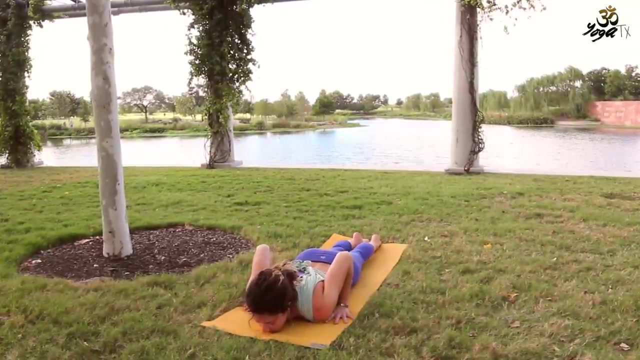 your hands to heart center. Take a few moments here, Kind of shift your neck around, roll your shoulders, Inhale up And exhale. plant your palms in front of you here for child's pose. Inhale. come forward And exhale. lower down slowly Inhale. take cobra So you can. 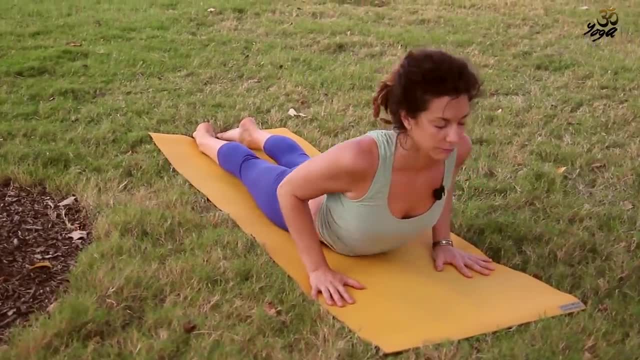 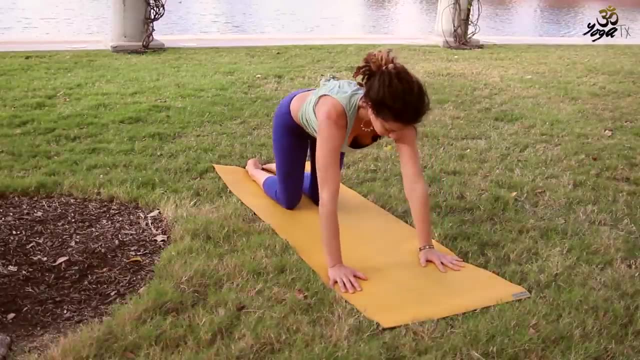 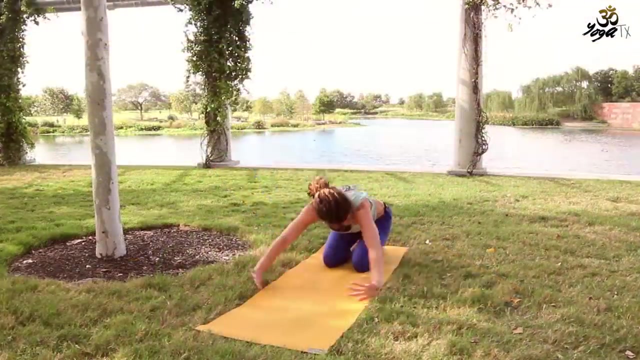 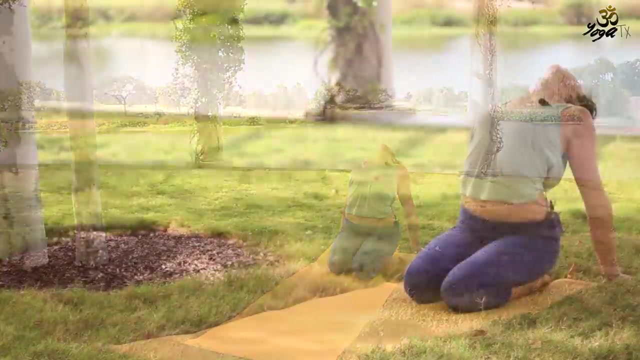 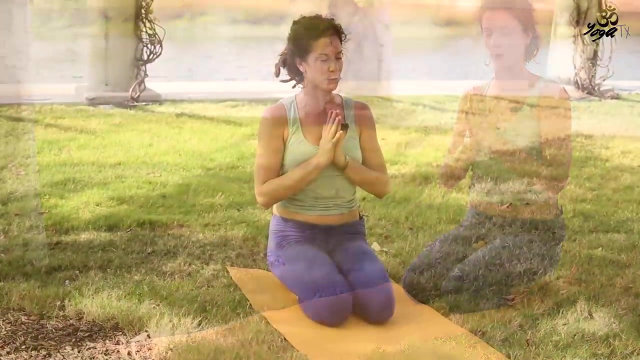 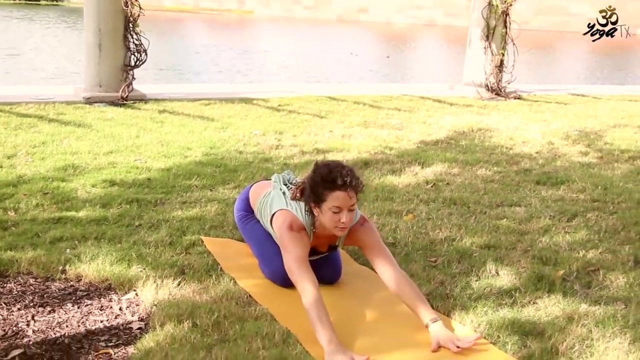 take low cobra, High cobra And exhale lower. Push all the way back to child's pose here, Bring your arms around And arch your back and look up And then come back to center. All right, So I'll take that a couple more rounds. So inhale And exhale child's pose, Inhale tabletop. 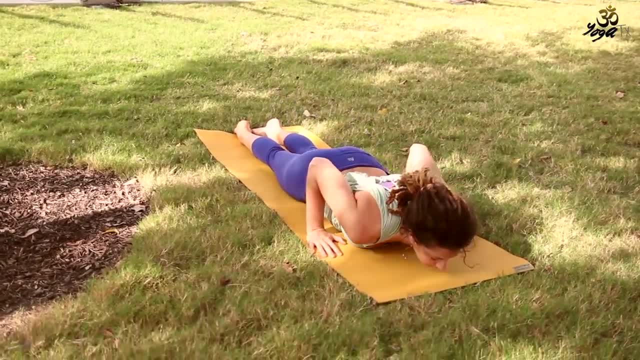 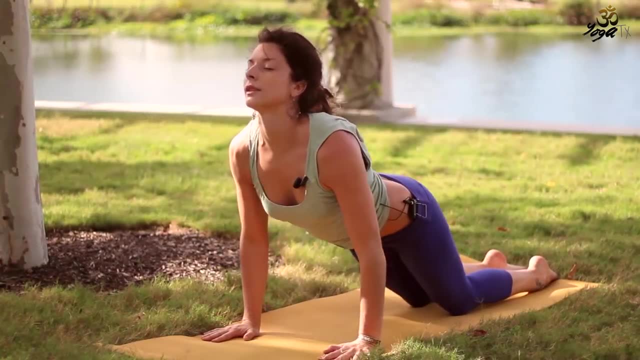 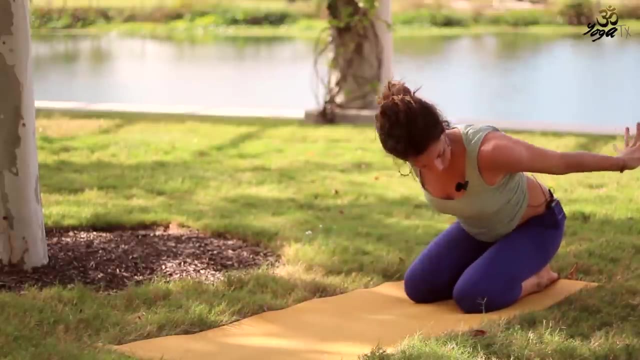 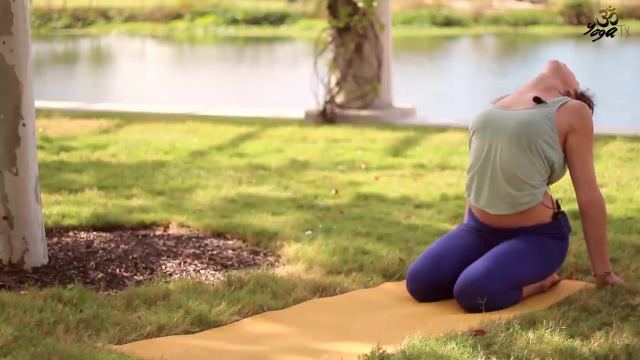 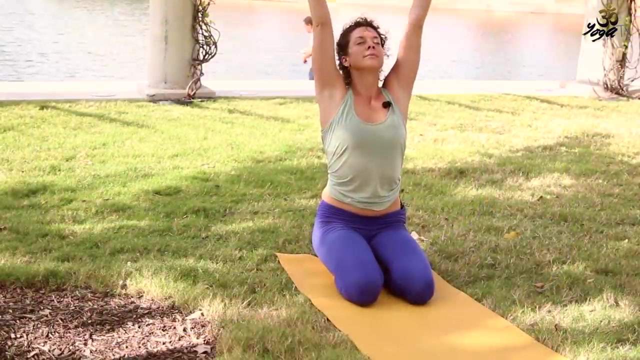 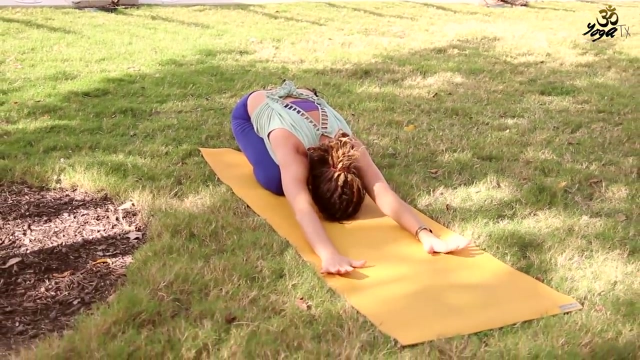 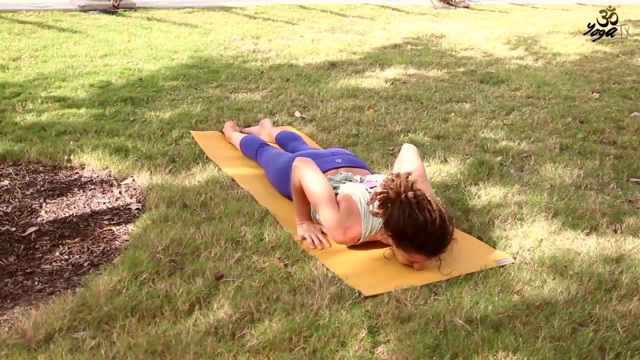 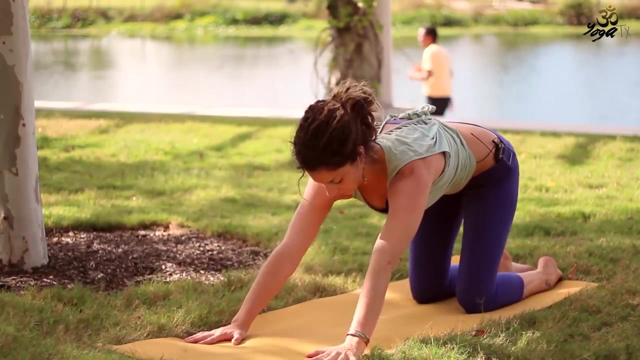 Exhale to the ground, Inhale, cobra, Exhale, child's pose, Sweep your arms around And inhale And come back to center, Shift forward And drop down And inhale. Try those sides again: Inhale, Exhale, Inhale. You can also come up Lift. 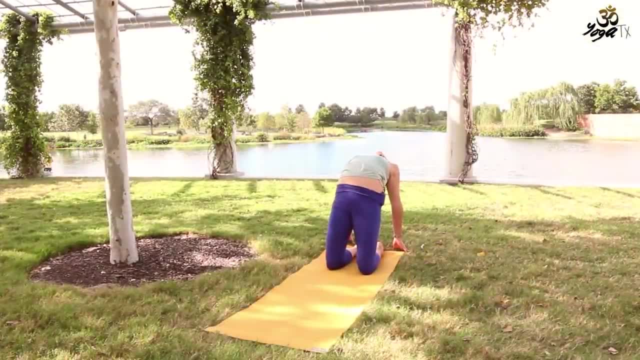 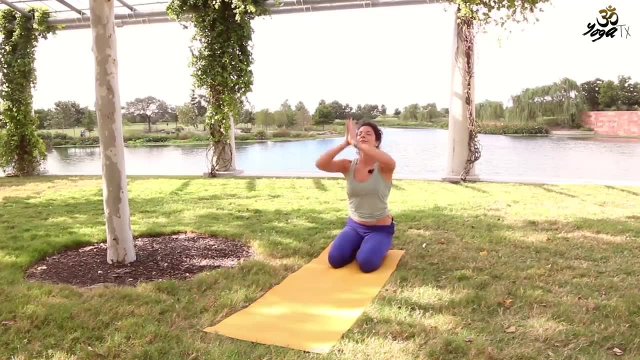 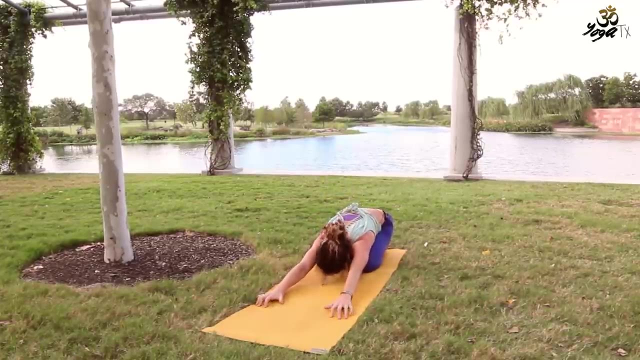 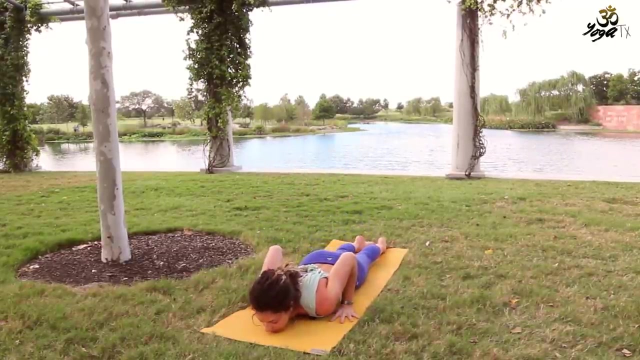 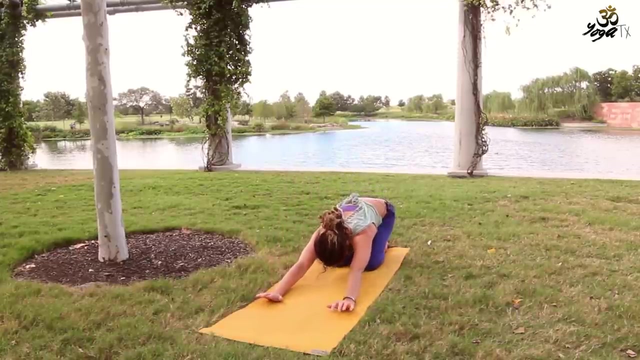 your hips up. You can also stay seated. We'll do that one more time: Inhale and exhale- fall. Inhale. shift forward and exhale- fall elbows in inhale. rise- exhale- child's pose- inhale. 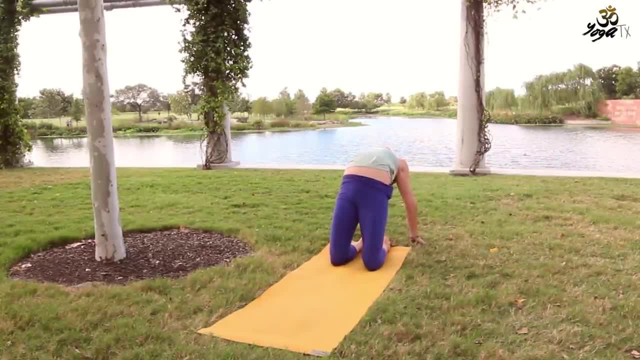 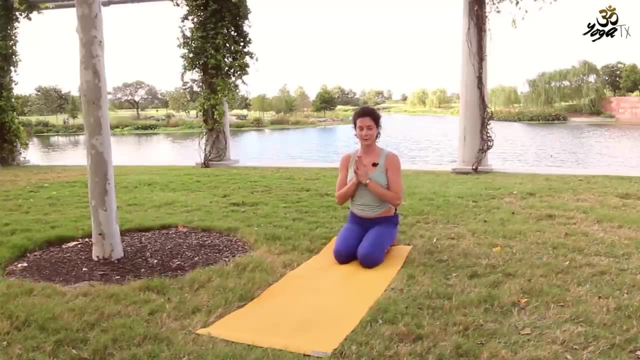 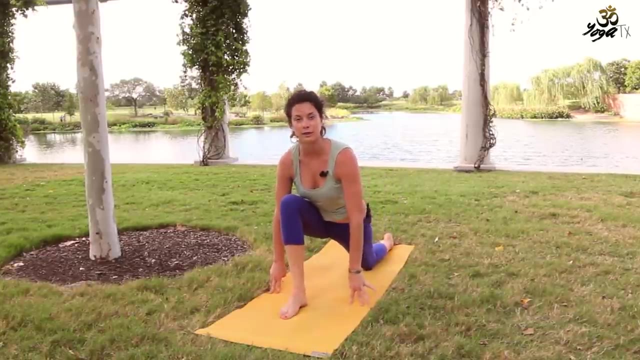 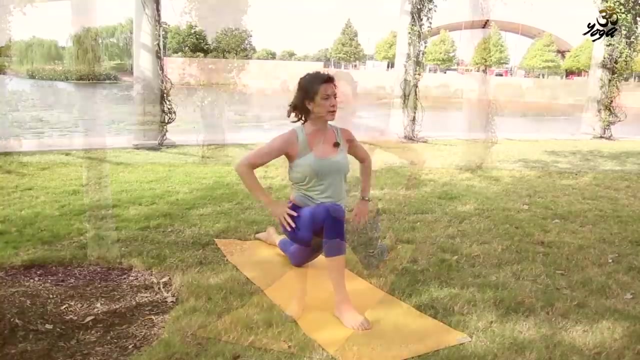 backbend variation. whichever, and come back to center. Wonderful, You're going to plant your hands here. We're going to take our right leg forward to a low lunge. Just sweep your arms up To help you find your balance. 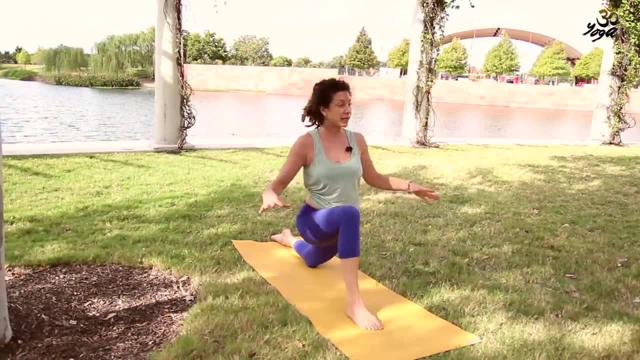 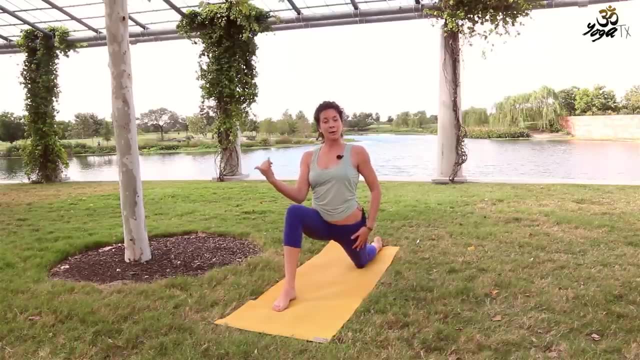 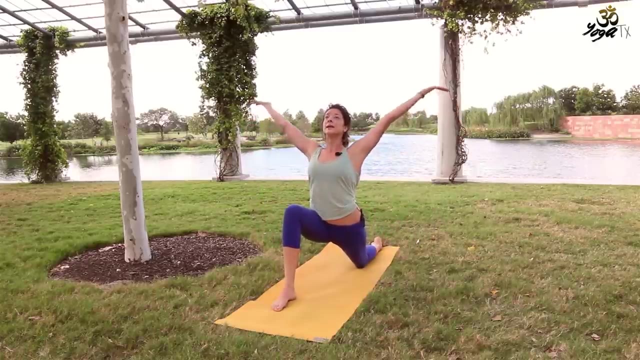 squeeze your thighs in together. That'll give a feeling of kind of sucking up. It'll feel like you're kind of rising a little bit and that'll help keep your balance. You can also shift this foot out a little bit farther to the side. That'll give you a wider grounding. So hands up, Bring your hands to center here. 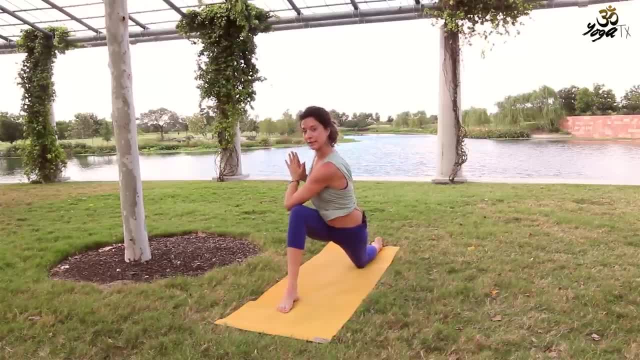 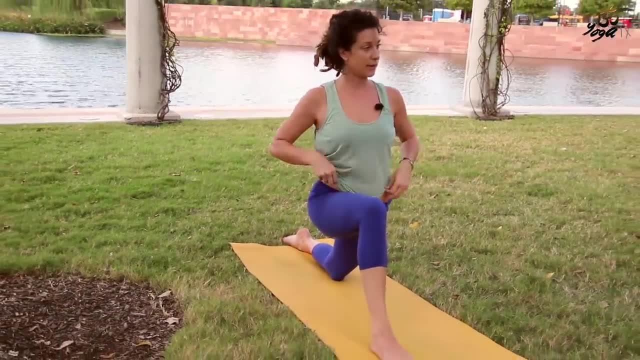 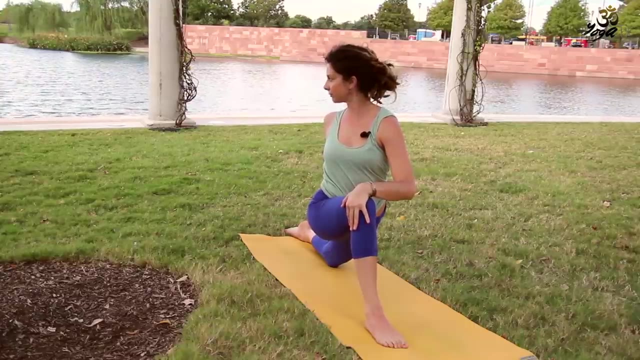 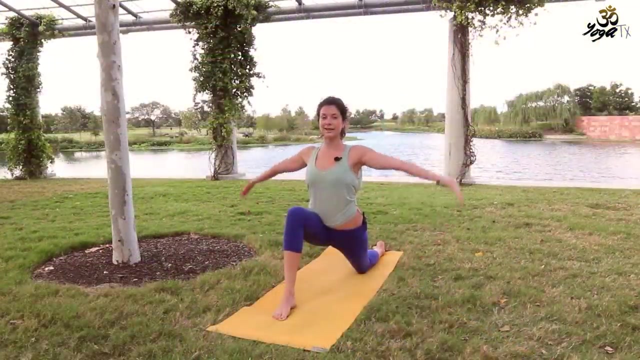 And if you can twist here, So left elbow to your right thigh, You could also put your left hand and just twist this way. I wish everyone feels more comfortable for you And inhale: come back to center, Drop your hands and we're going to straighten our front foot. 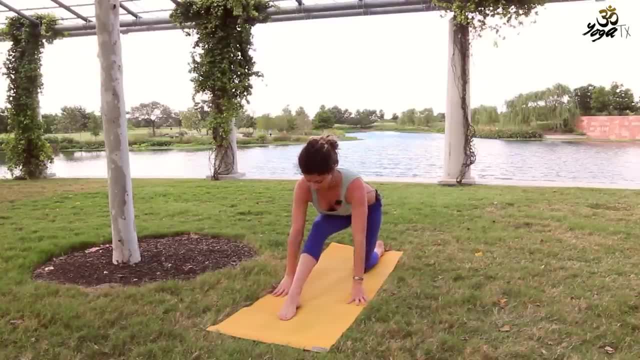 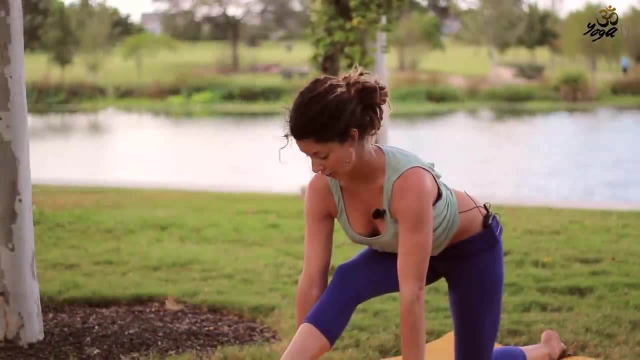 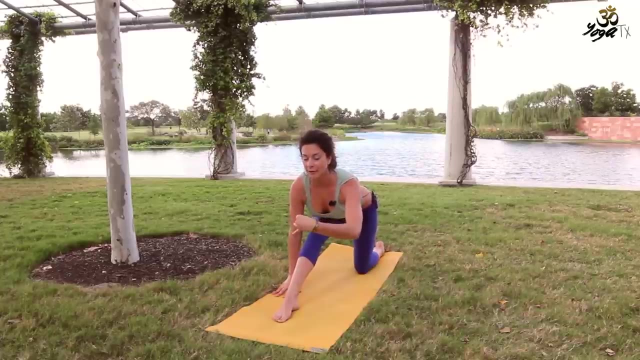 You can keep this leg bent if you need to. We don't want to round over, We want to keep our back straight. So if that means you stay right here, then just stay up. You can stay up with your knees bent. Mine's a little bit bent here. You want to have the feeling of extending out from. 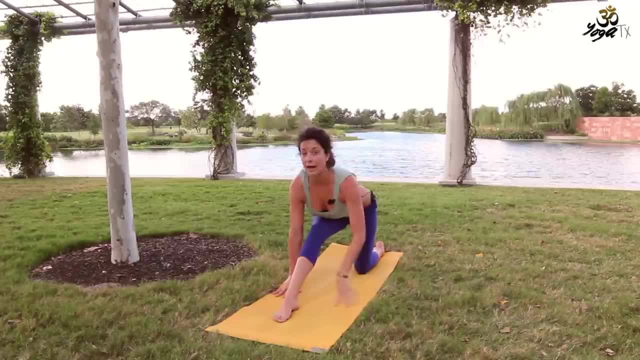 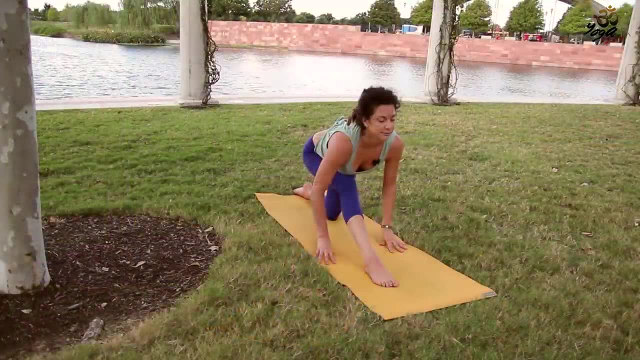 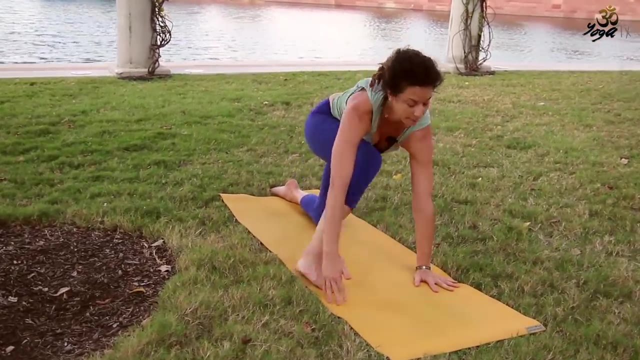 your pelvis, So actually coming forward instead of down And then see if you can come down a little bit. Shift back forward, Plan our hands and we'll come back, and we'll do that on the other side. So bring your left leg up, Find your balance, Put those hands here. So if you're feeling a little bit, 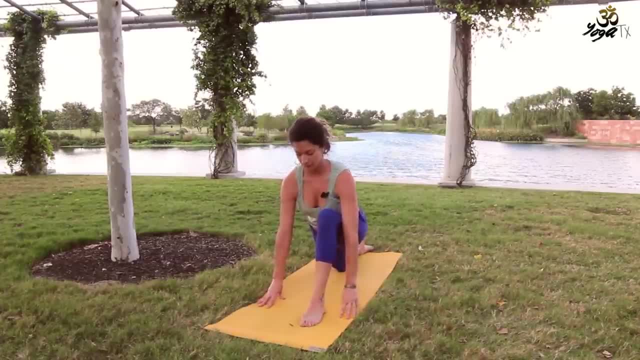 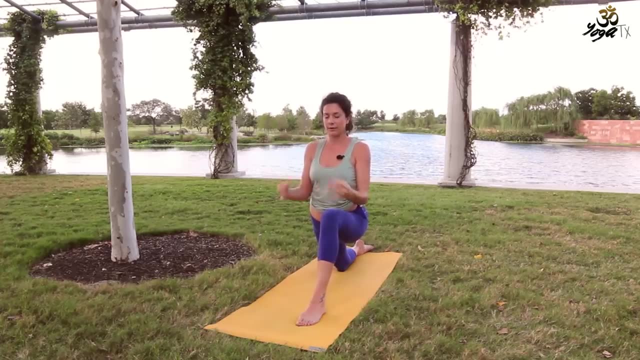 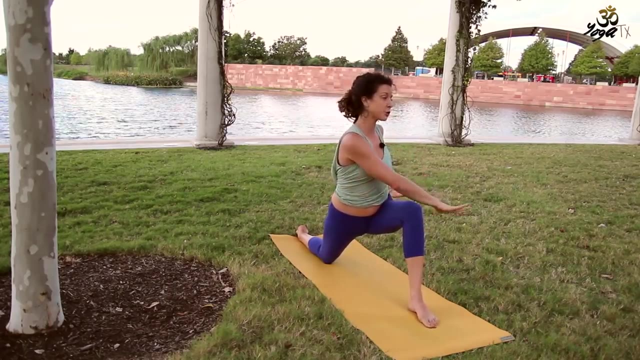 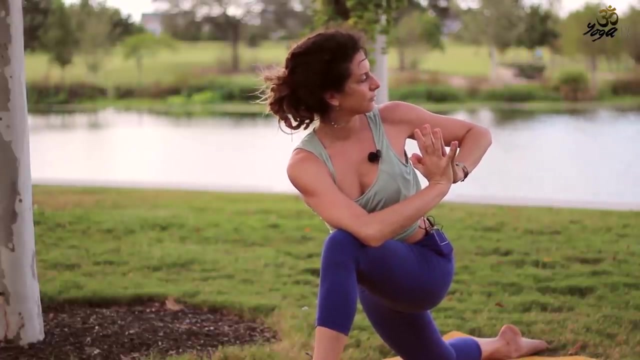 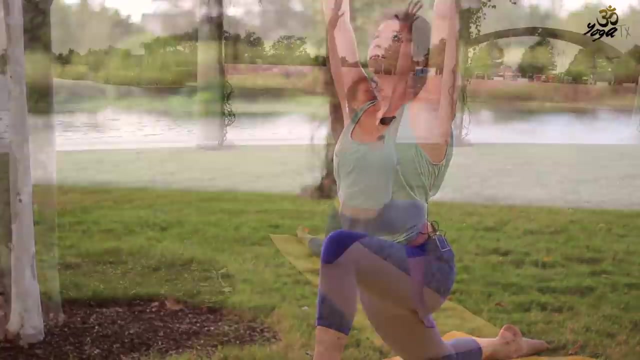 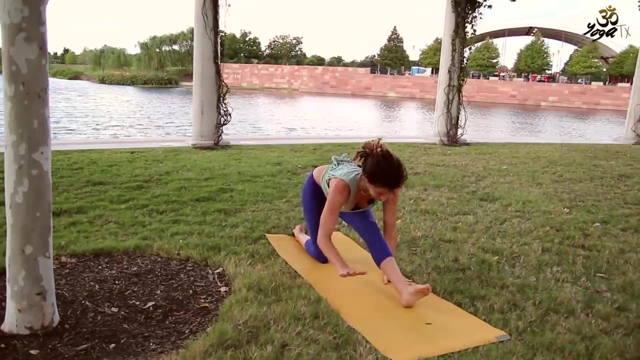 balance here. You need to bring your leg out a little bit And rise, Suck your inner thighs in, together, that feeling of coming towards the midline, And we'll take our hands to center and take the twist, whichever version. Come back to center Your hands And again, extend. 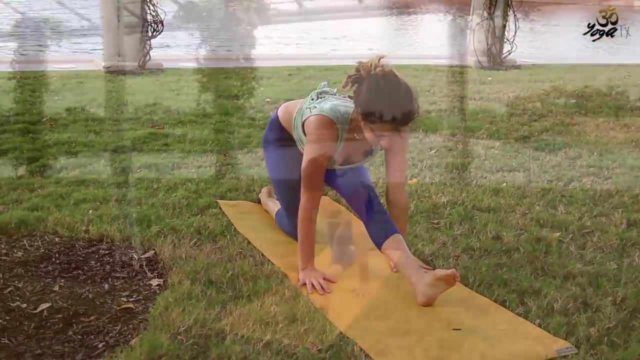 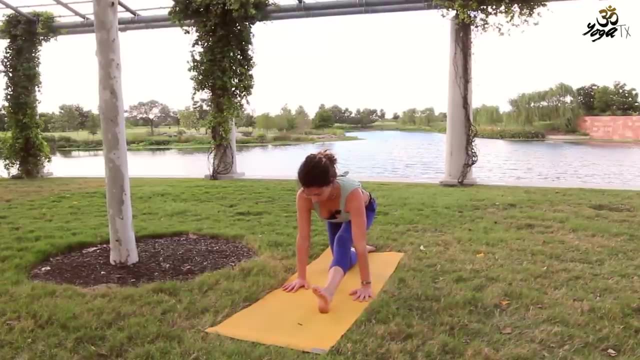 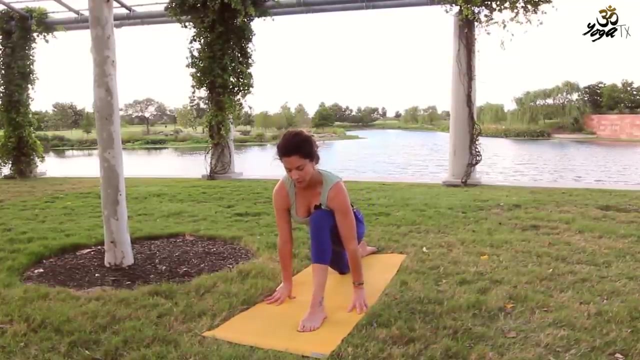 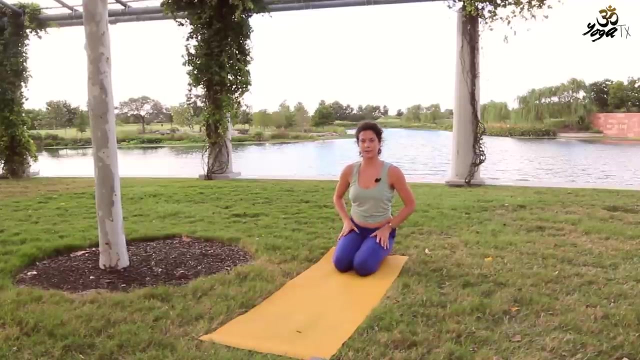 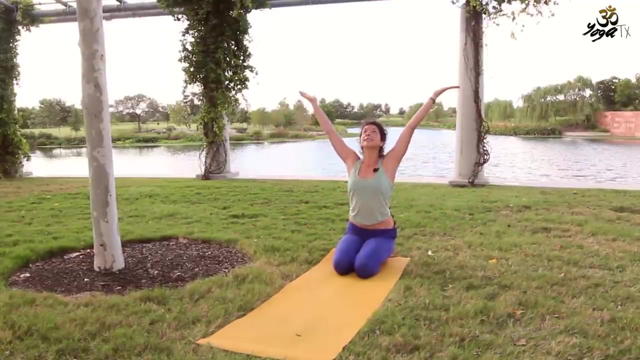 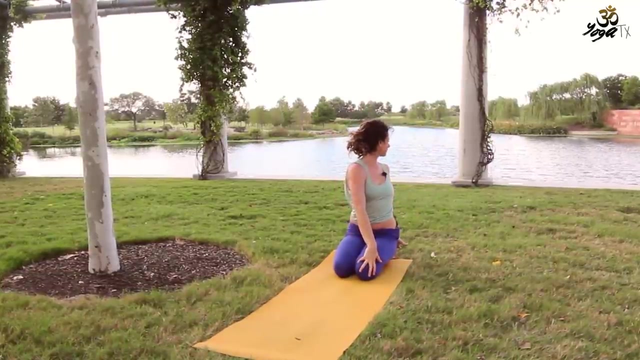 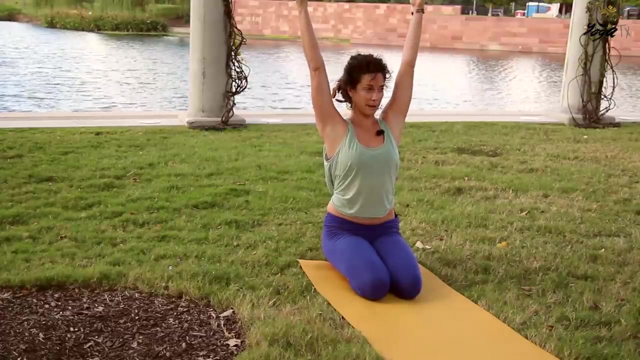 out before you come down. Come back forward And step back. Come back to sitting on your hips here. Let's take another little spinal twist while we're sitting right here. So come up And again twist to the left. Twists are wonderful for back pain. It gets all those joints, the fluid. 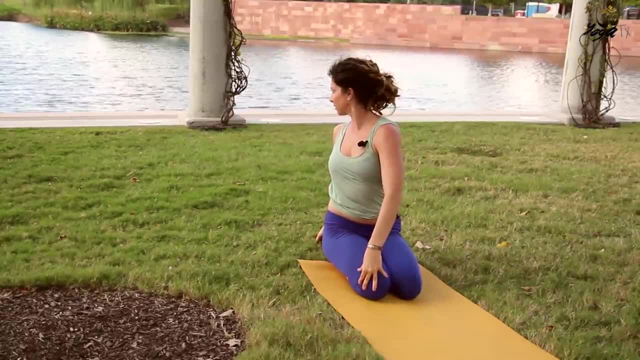 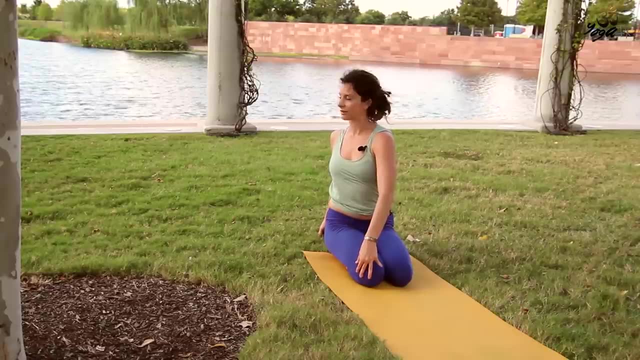 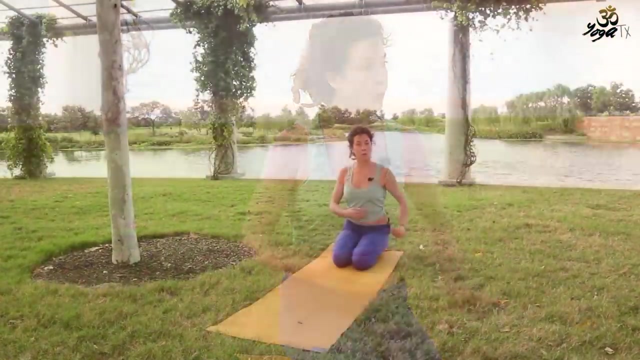 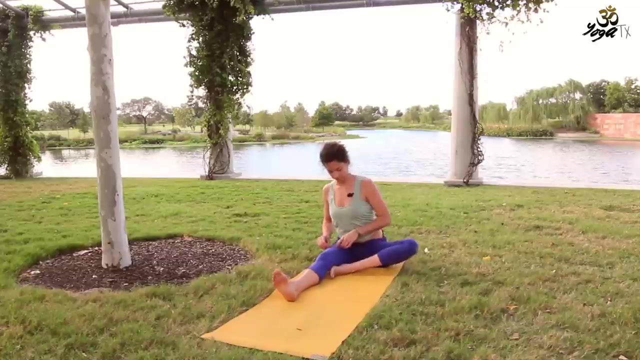 the synovial fluid moving Around which helps fight the stiffness. Okay, And from here, just roll over to one side of your heels. We're going to bring our right leg out in front of us And bring your left knee, if this is available to you, in to your 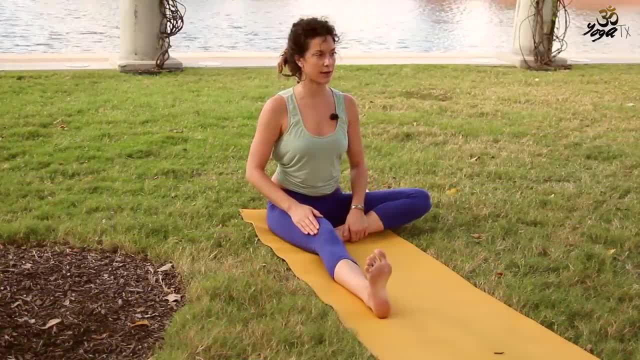 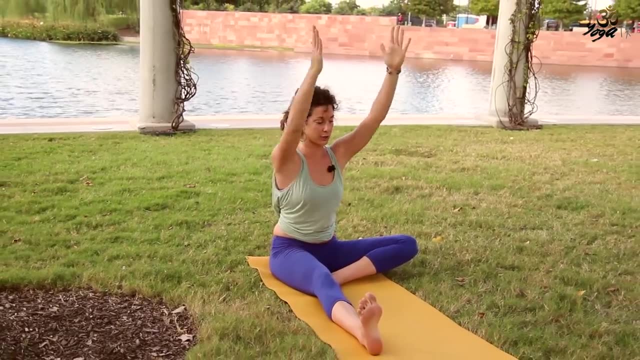 right thigh. So we're going to have our right leg coming straight out. We're going to bring our arms up and shift your torso over your front leg. So you're not coming down right here. You want to be coming this way. So inhale and on an exhale. 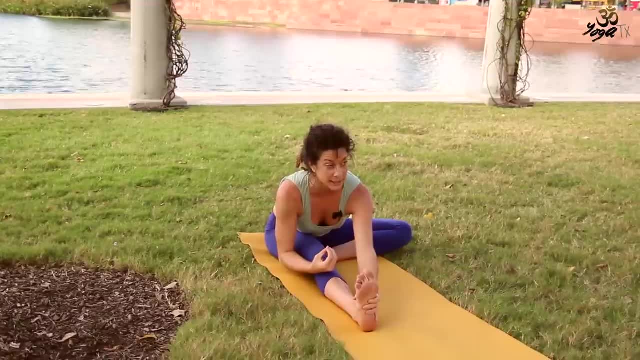 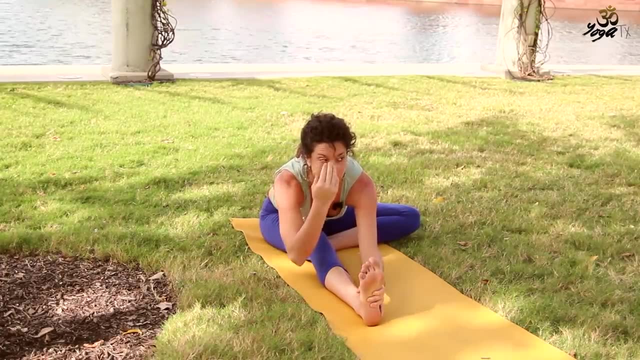 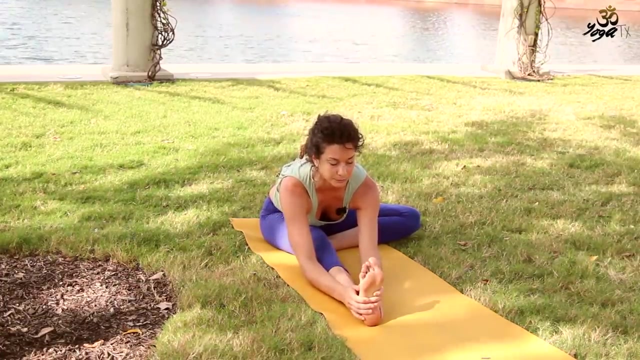 Come forward And again, like we were talking about, like I was talking about, you don't want to be coming down. Think about bringing your head to your foot and then come down. You don't want your back to round. So the extension is the most important And this: 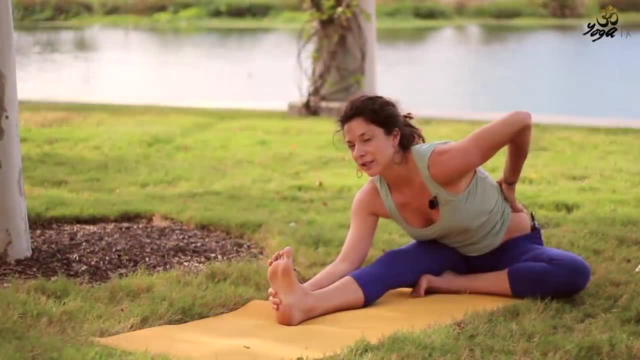 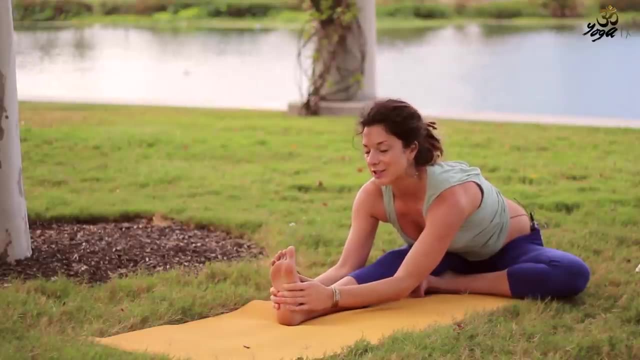 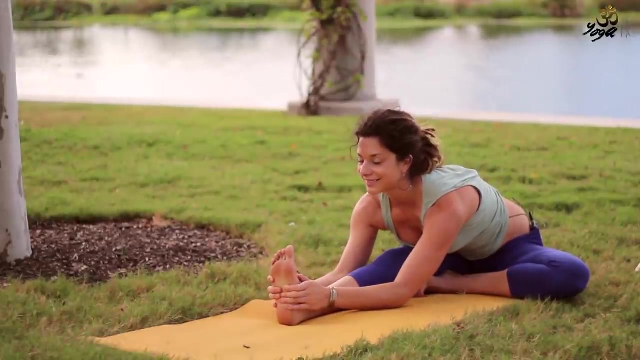 is great. I can feel it on my QL right here. This low, one of the low back muscles really, really needed this stretch. So again, you can inhale and extend and exhale, Sink down. again You can let your head hang. 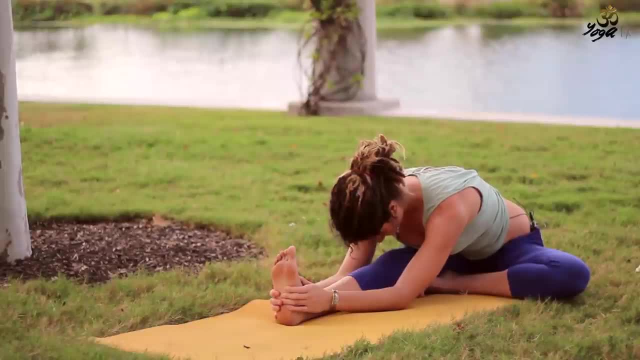 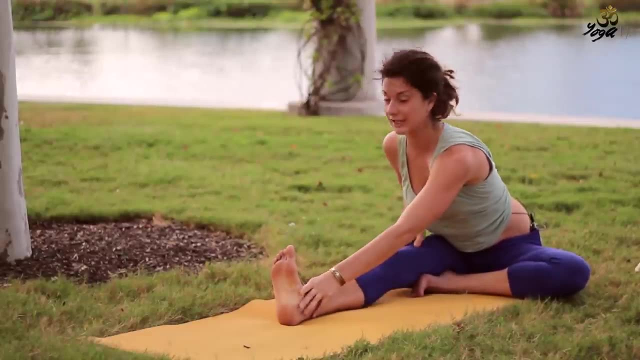 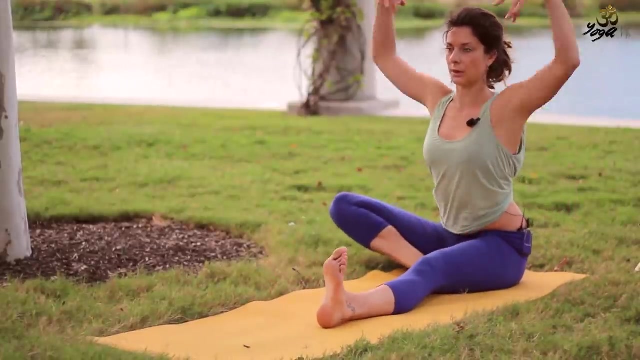 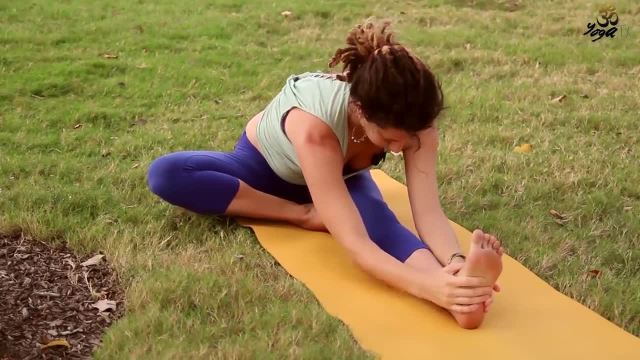 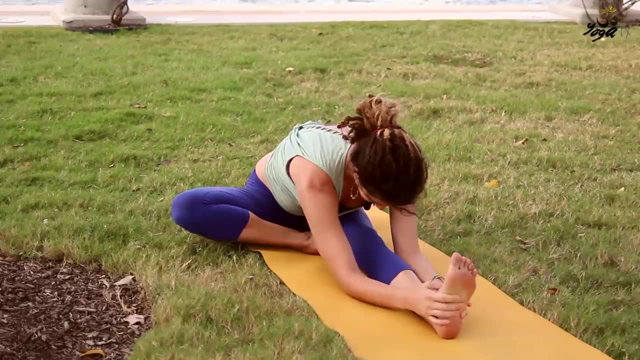 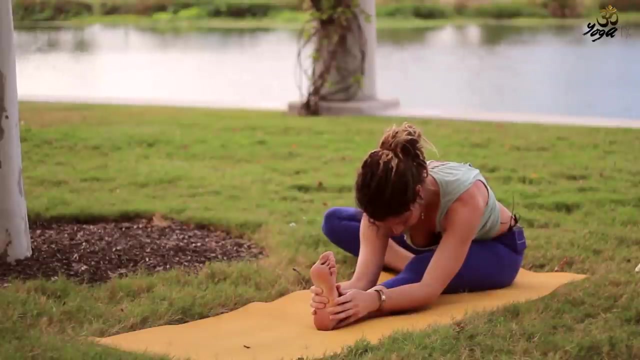 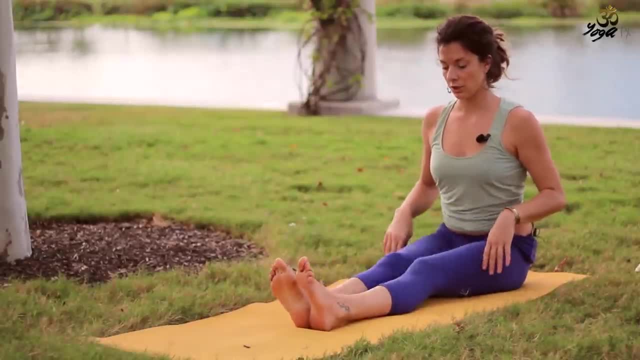 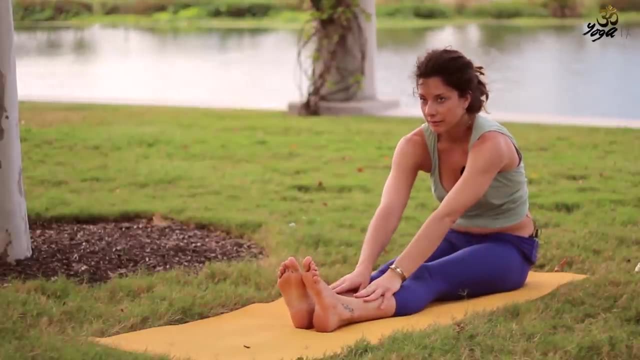 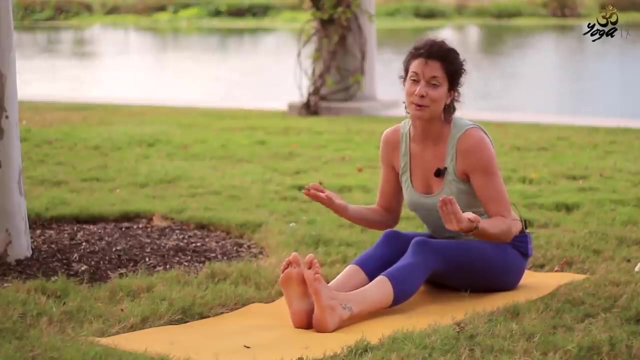 We'll take it with both feet out So you can bend your knees here if you need to. We don't want this. So if you, if it's better, if you need to bend your knees, then do that. You want the extension in your back more than the hamstring stretch for the purpose of back. 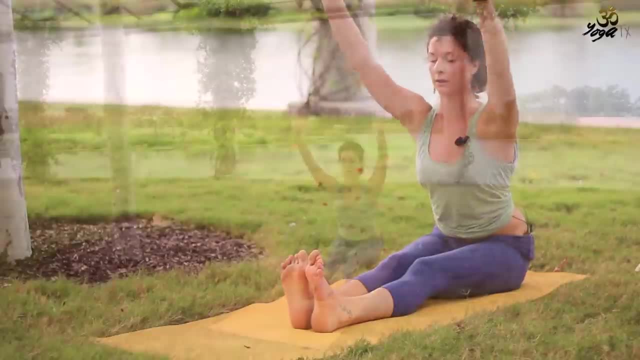 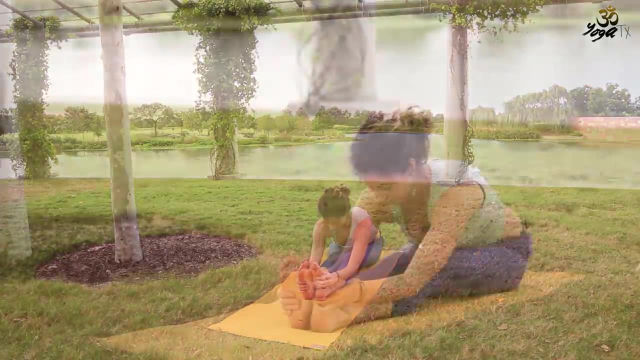 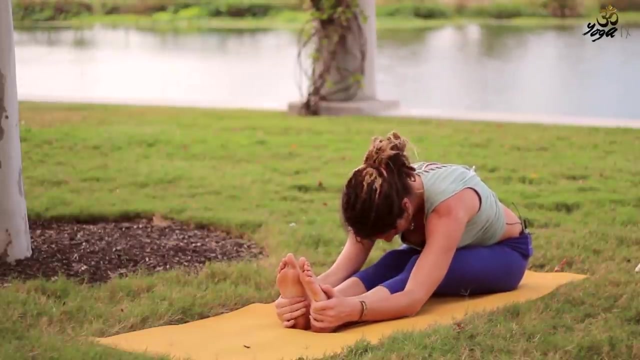 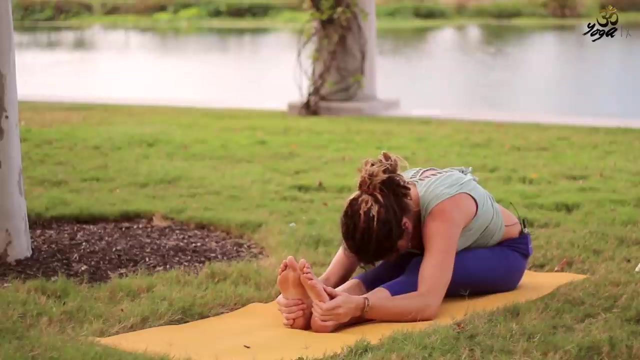 pain. So inhale up and exhale over. Release your head here. Okay, So we hold our head up all day long, so just that in itself can cause a lot of neck pain. So just release down to the ground, Extend your spine and fall one more time. 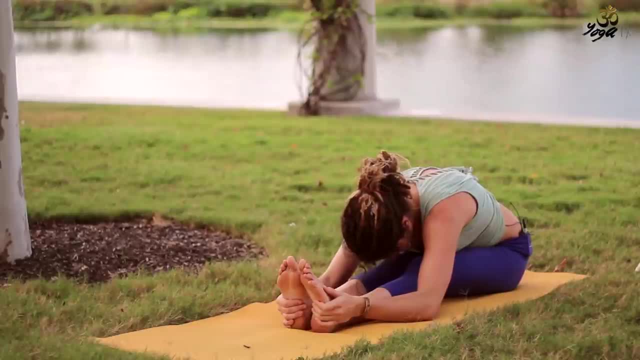 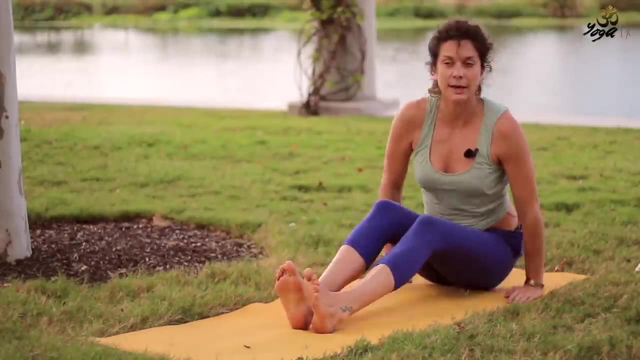 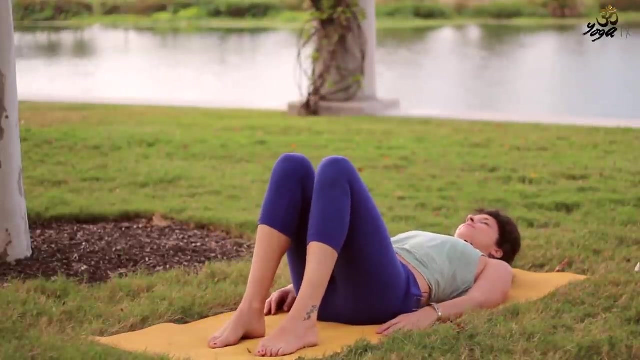 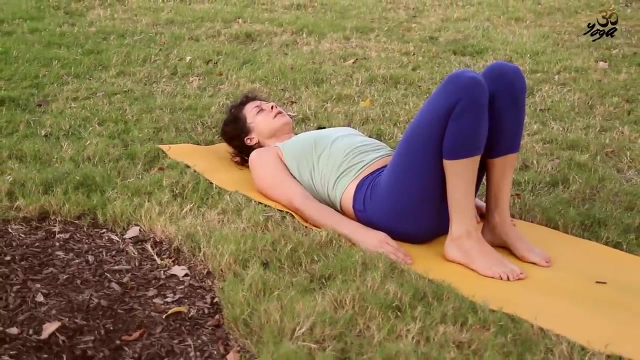 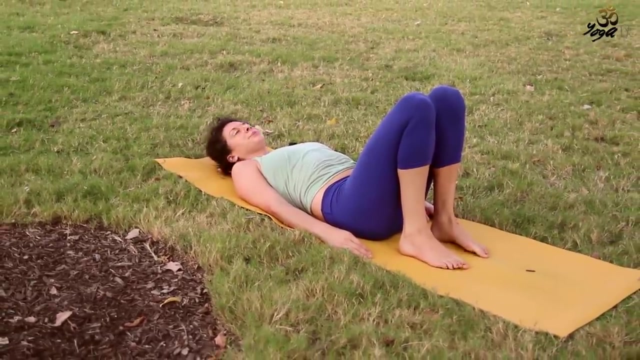 Okay, Rise back up. So go ahead and come to laying on your back here and shake your hips out a little bit. We're going to take one bridge pose, Kind of traction: the lower back out. Okay, Good, Good. So bring your heels to where you can touch them with your hands. 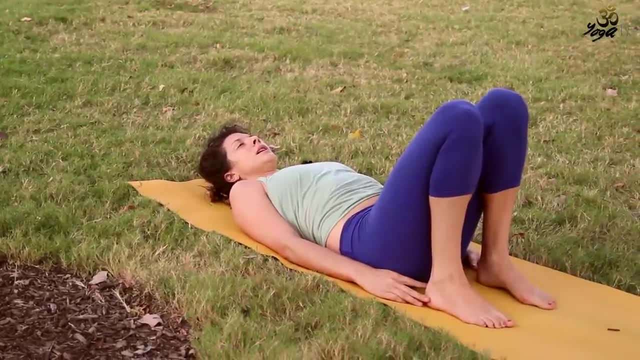 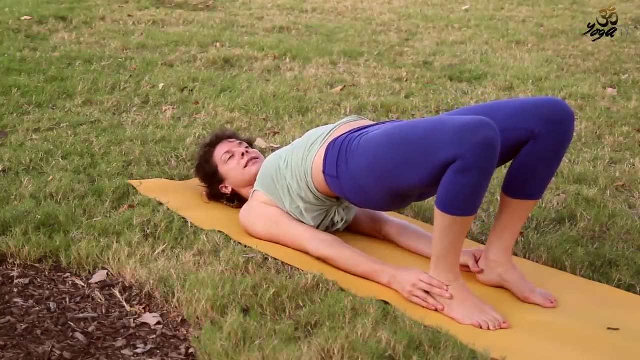 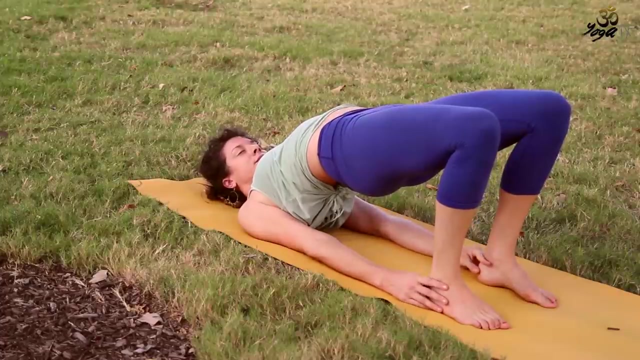 You're going to slowly raise your hips up and, as you do, roll your shoulders onto underneath your back and then lift your hips up farther. This is another really good back strengthener. You want to try to release your glutes here and try to use your back strength and your 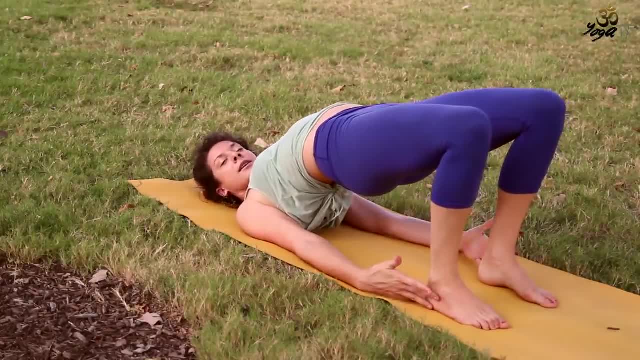 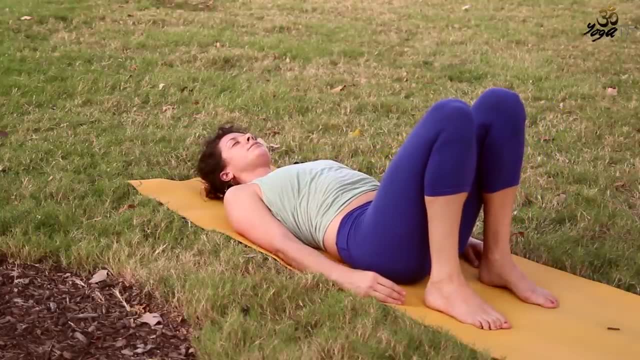 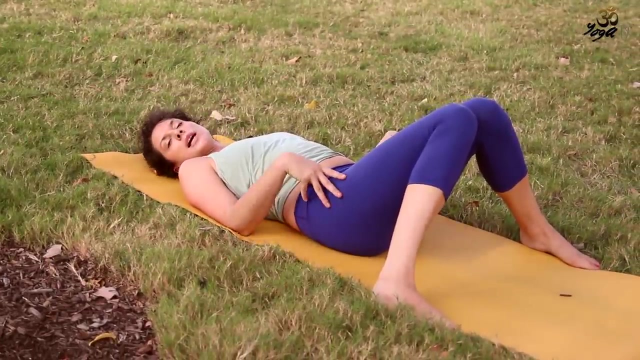 quad strength. Lift your hips a little bit higher, Inhale And go ahead and come back down and untuck your shoulders. You can bring your feet wide and let your knees fall in. This will neutralize your hips, this position here. 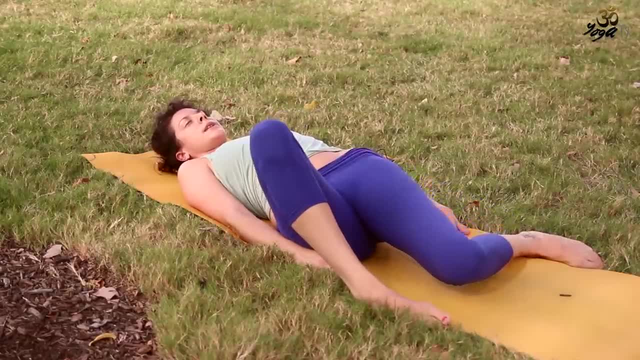 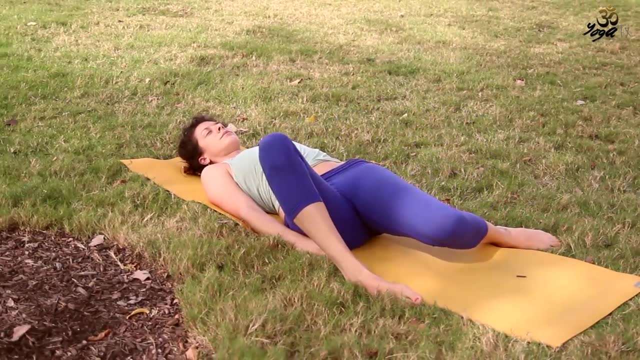 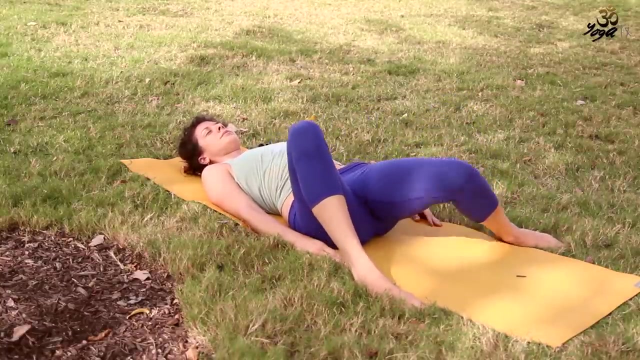 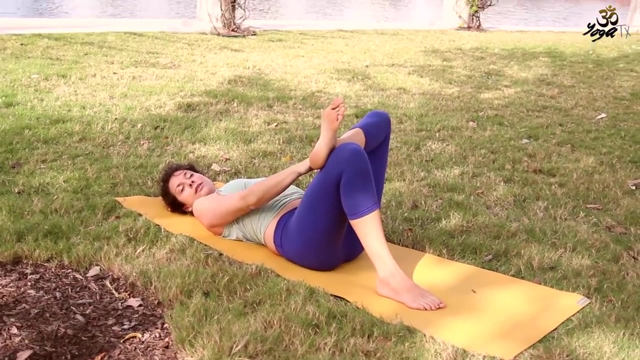 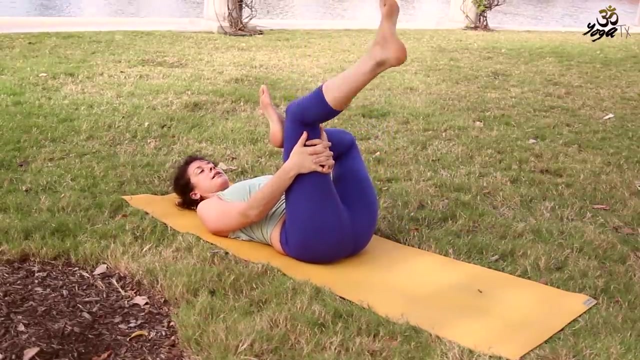 Go ahead and let them windshield wiper from side to side- Good, Good, Good, Good. And bringing it back parallel, we're going to take our left heel and take it over your right thigh And come in and grab the back of your right thigh here. 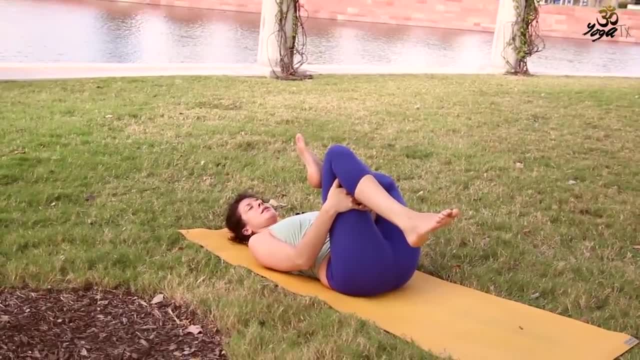 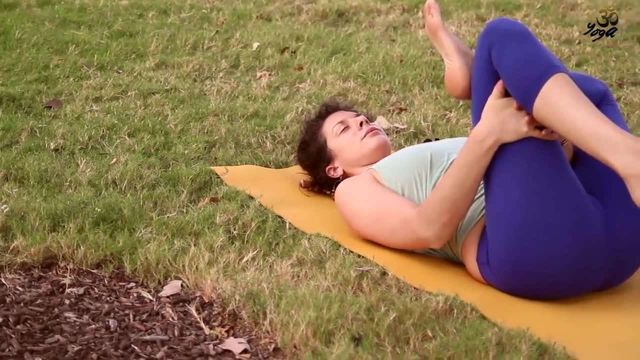 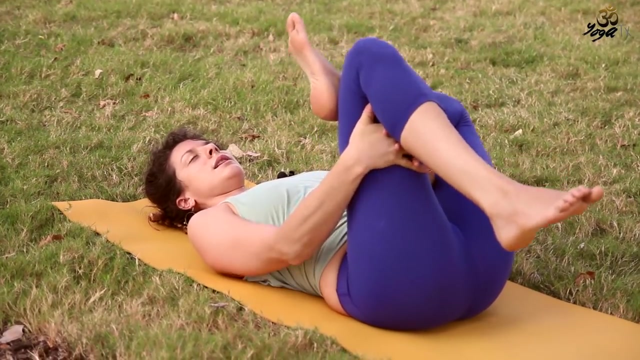 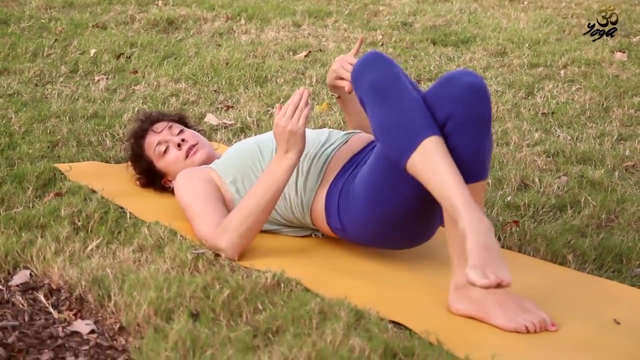 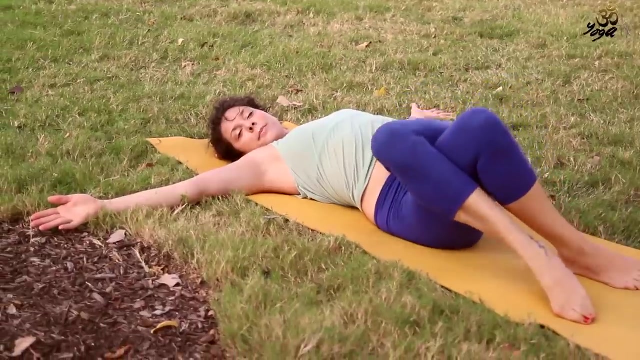 Just going to pull in Good And release your right leg, Cross your left leg all the way over. We're going to scoot our hips over about three or four inches. put your hands out to a T, drop over to the right and look to the left.